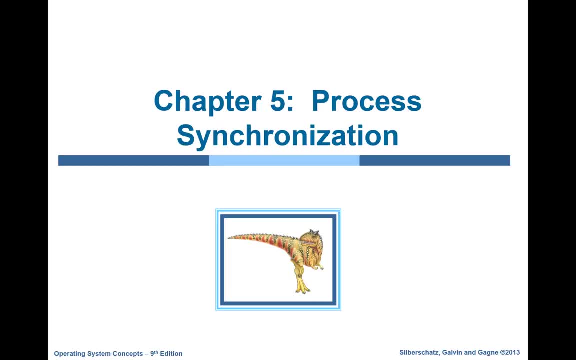 okay, bismillahirrahmanirrahim. so last time we started chapter 5, process synchronization, but because the projector was not available, so i start again. okay, briefly, we will revise what we studied last time and then we will move next. so, inshallah, today we are going to finish this. 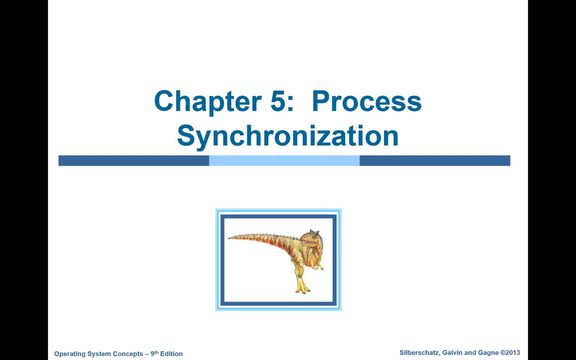 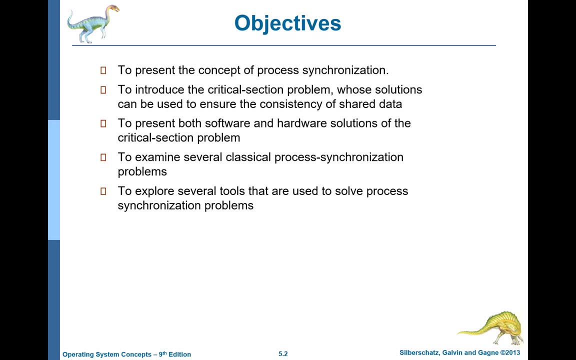 chapter 5, which is about process synchronization. now, what we will learn in this section is the concept of process synchronization. we will study about critical section problem, okay, and then the solution, some of the solution. there are some solutions which are software, some solutions which are hardware, okay, and then at the end you will see some classical process synchronization problems. 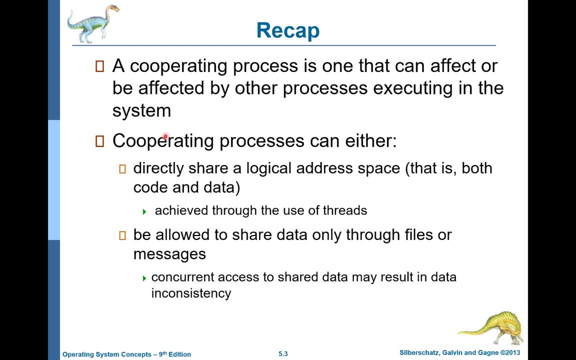 okay. so the first thing is we have a recap from chapter two. we revise from chapter two, in which we studied about cooperating processes. okay, so a cooperating process or group of operating processes are the one in which the processes, they affect other processes or they are affected by the other processes. so any process can be cooperated if it can. 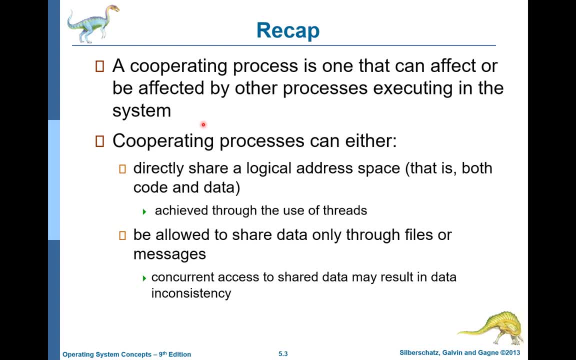 do some change, some influence on the other process. it can give something, it can send a signal, or it can receive something or receive some signal, etc. okay, so there are different reasons for cooperating processes that we studied in chapter two. now cooperating process: there are two possibilities that we have. 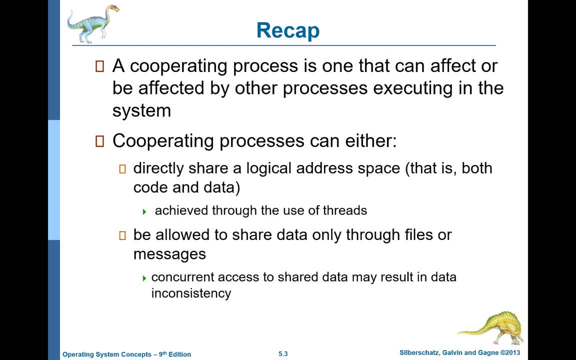 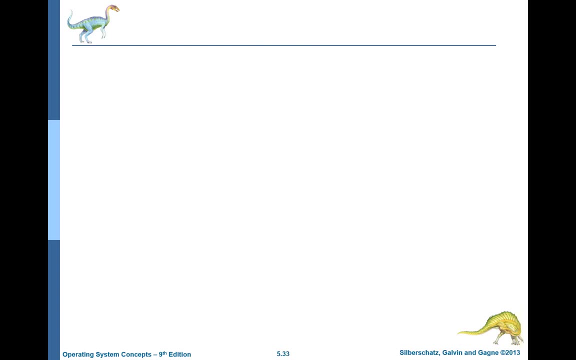 discussed, you know, inter-process communication. one was about shared memory and the other one was about message passing. so, in case of shared memory, if you remember, okay, let me draw this diagram. if you remember about- uh, just wait, give me one minute. if you remember, we studied that. 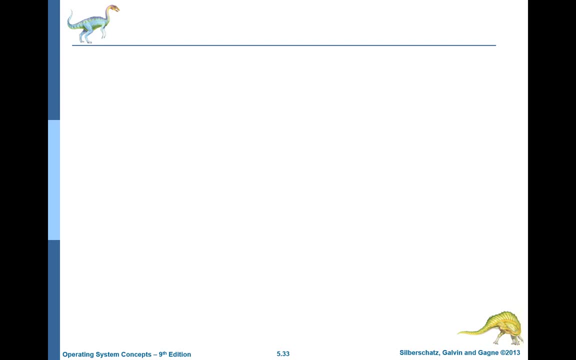 what we had. a process in general. let's say, this is some process in memory, okay, so this one process. the idea is that it has sections. it has data section, okay, if you remember. it has this heap and data and text, okay. so there was text or code. and then there was, uh, let's say heap, okay, and it can be anywhere. so there was a heap. 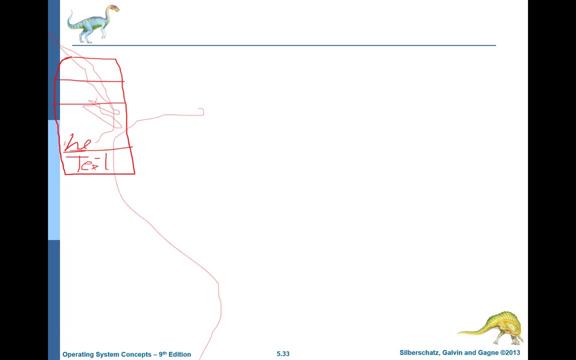 sorry, i locked it. just let me give me one minute. it is there, okay, okay. uh, so what i have is: there is a heap somewhere. okay, this is the heap. oh, very bad today, i'm not, you know. okay, so this is the heap, heap, okay, which can grow. then we can have the data, okay. 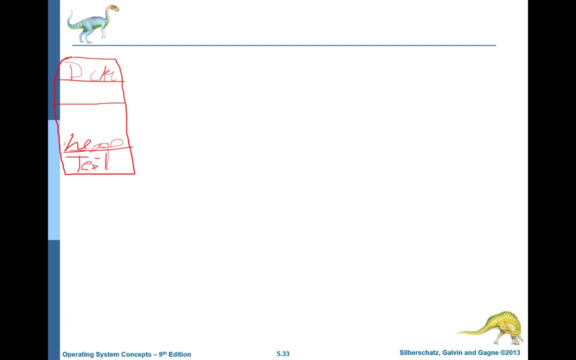 other stack. um, okay, so these things grow. i'm my writing is very bad on the computer, but anyways. so this is a single process, okay, what we have in case of multiple processes or, sorry, a process which has threads. so this is a process, okay, which can have two threads, for example. so we divide this. 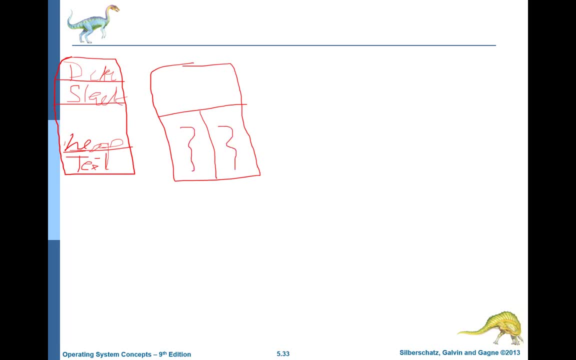 just visually to show that there are two threads of this process. okay, so these threads, each one has something which is its own, which is a stack, so each thread has its own stack. that was what we discussed in chapter four, in the last chapter, and then actually they share the data and the heap and 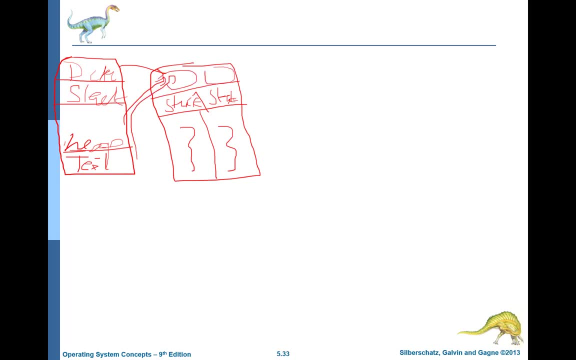 the text sections. they are shared between all of them, how many threads they are. so this is the general concept of how you share actually the data or the heap between the tracks. okay, so threads can help in shared memory. the other was about message passing and in message passing, if you remember. 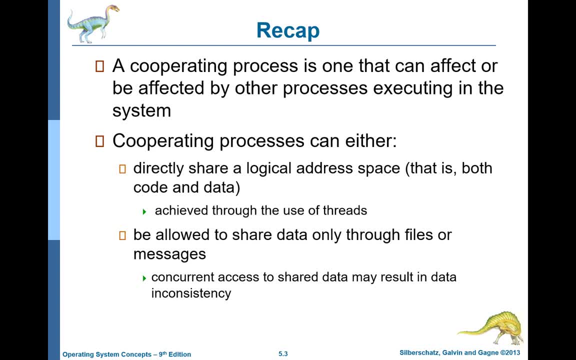 we have two processes which which pass messages to one another, and this involves actually the operating system kernel, which is responsible for passing the message from one process to another process. now what happens is that we we see that if you have concurrent access to shared data, okay, why share data? because it is shared between two or more processes at the same. 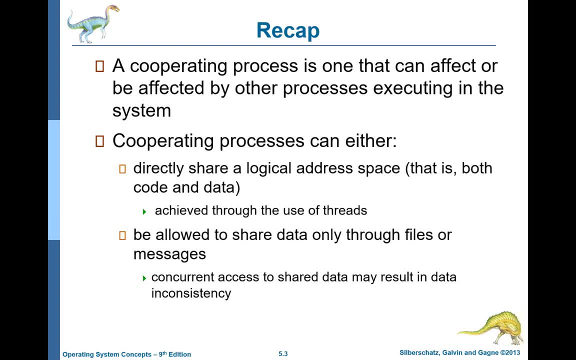 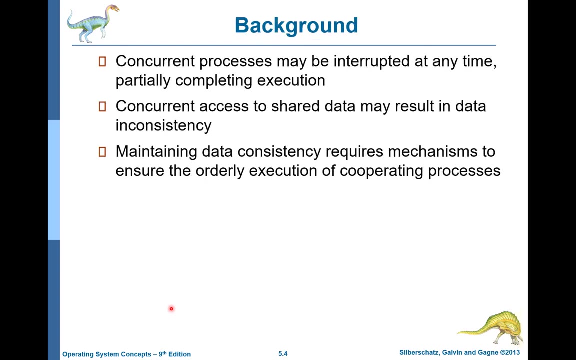 time, then it can result in data inconsistency. okay, and what is data consistency? it means that the data variable can have different values for different processes, or it can result not in the correct values, which is except expected from that. we will see this example of data inconsistency later on. so why does this data inconsistency comes into play? 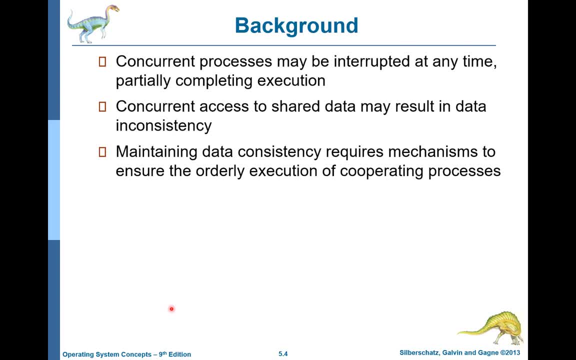 because the main problem is that you know context switching, okay, or multitasking. so when a process is running on a cpu and because of some reason the cpu is taken from the process, so this is an interruption, okay, so it does not complete the execution of the process. the process is in the 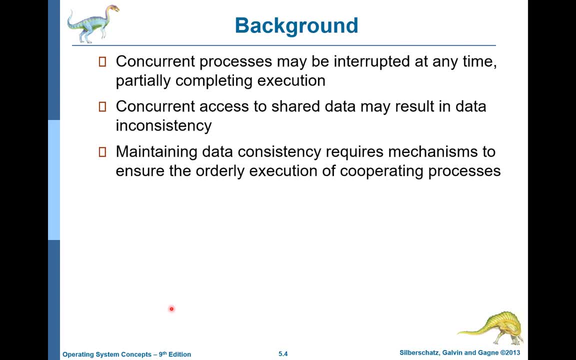 middle of doing something. if the process was modifying some data and it was interrupted, it's possible that the data becomes inconsistent. it is not in the stage which the process wanted before the completion, so it wanted to change the value of the variable, but it was not changed, and when the other process comes, it 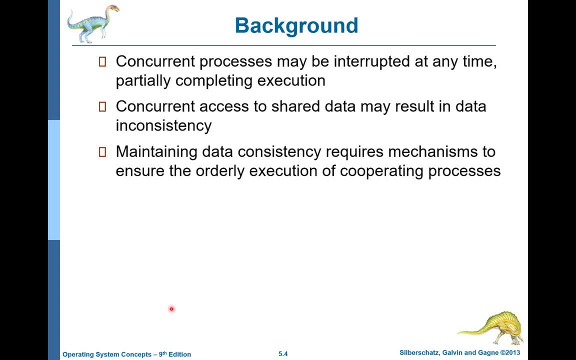 accesses the same variable and it finds old value of that variable, which results in inconsistency and the application has some error or some problem. okay, so that's why we maintain data consistency and we want to execute these cooperating processes in some order which will ensure the consistency of the data. before that, let's understand the producer- consumer problem. 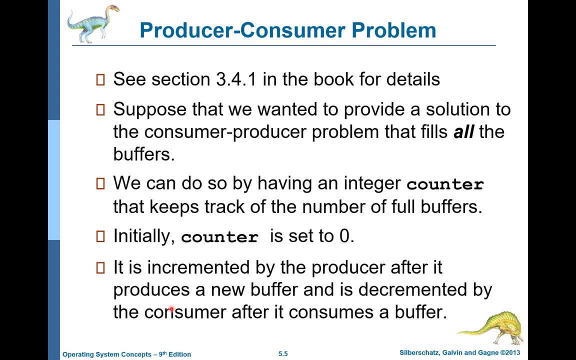 now, what is producer consumer problem? we can see the detail in section 3.4.1 the book, which is about shared memory or message passing. okay, you should go and study that section. okay, and then you will understand the producer consumer problem. okay, so there are different types. 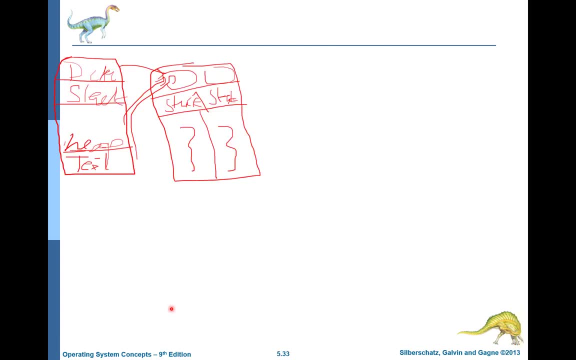 of discussion on producer consumer problem, but what i am actually telling you now is just an explanation of one thing which is the bounded problem of, uh, consumer, producer. okay, so let's suppose you have a buffer. what is a buffer? you know? a buffer is some memory space. so here let's say, i have this buffer, this. 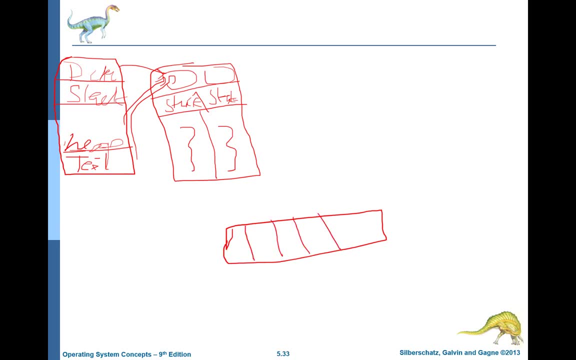 memory and it can be considered as an array. okay, now it has some positions like from 0, 1, 2 until max, or buffer size. okay, so this max is actually the buffer size, so it can be 10, it can be 100, it can be million, whatever it is, but these are different positions in the buffer, so let me 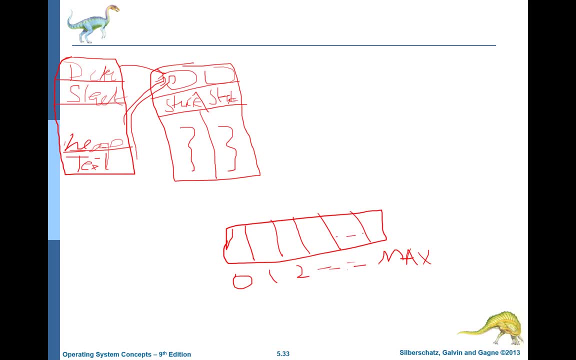 make it like this. now we have two processes. one process is called producer process, which produces something into the buffer, so it will write something into anywhere in the buffer, and the other process is the consumer process, which will actually read something from somewhere in the buffer. now the producer it produces and you see, the buffer has some bound or some limits. okay, 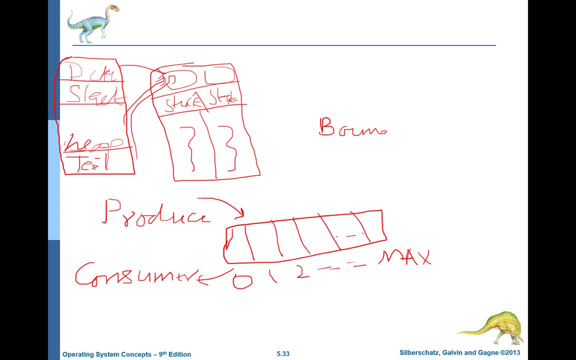 so this buffer is bound, bounded, which means that it has some size and it produces. the producer keeps producing something, okay, then after some time this buffer may become full, okay, so this is one thing. the second thing is, if the producer is slow and the consumer is fast, then it's possible that the buffer is empty because the consumer has 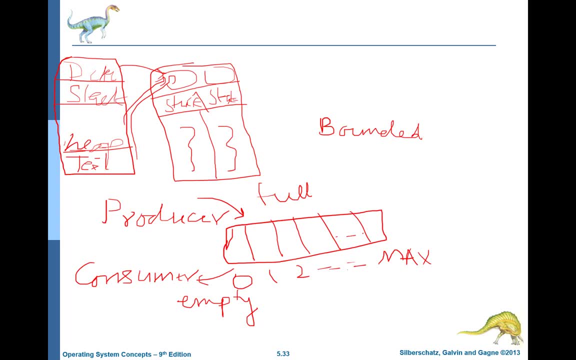 already consumed all the things and the producer has not produced enough. so these are the things you need to see now. there are three things we need to remember. one is the pointer which is called the in pointer, which means when the producer produces something, so actually it will see where to produce. 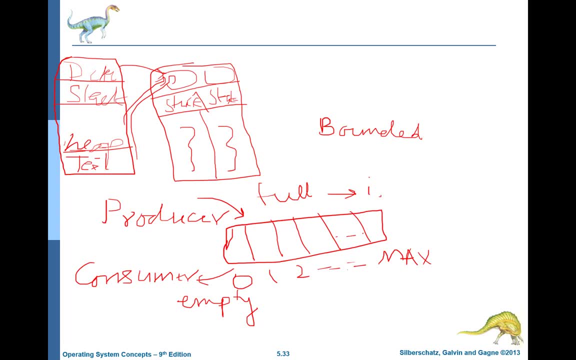 that thing. it will use the IN pointer. the IN pointer will actually contain the, the location where the producer may produce something. so maybe that initially the producer produced something in here. for example, it produces some number, let's say it says 10 here. okay, so the in is here. then the in will come to this position 1, then it. 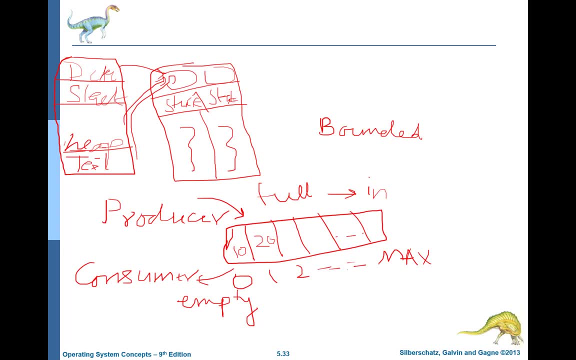 says 20, okay, and after that let's say it says 5, so it has produced three numbers in these locations. and the consumer it has a pointer which is called the out pointer, and the out pointer actually it points to the location from where it is going to consume. so let's say in the start: the out pointer is here, okay, so it. 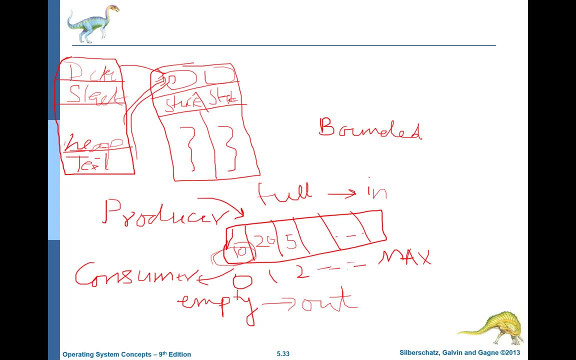 will consume number 10 when it consumes. so, beginning in the beginning, there was three numbers, but when it consumes this one, the out will come to 20 and there will be two remaining items in the buffer. okay, now the thing is that if the producer consumes until the end, okay, let's say the max is 10. 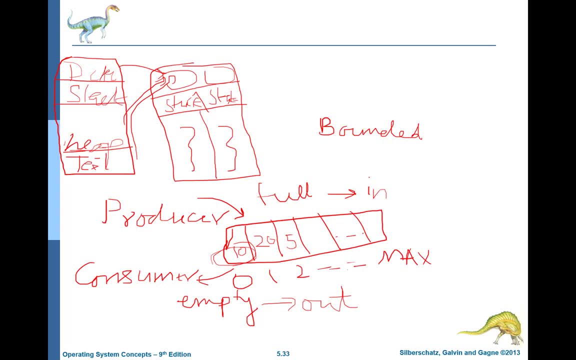 and the producer wants to consume more and the consumer has. the producer wants to produce more and the consumer has already consumed half of it. so this area, which the consumer has consumed, will be free because the consumer is here, in this area. okay, sorry, the consumer is in this area and this area is free and the 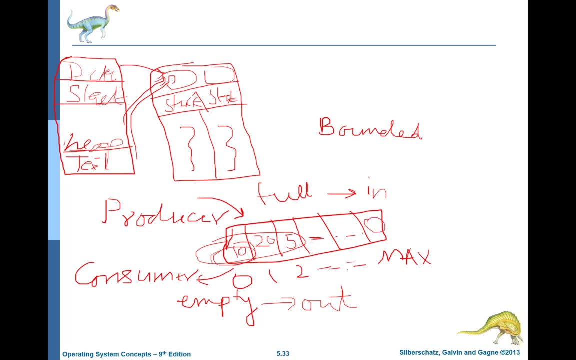 producer is here. so what will happen? how do we know? if this area is free, what should we do? when the producer comes at the end again, it will start from zero and it will keep producing in these areas, one by one, okay, and the producer will be moving forward. 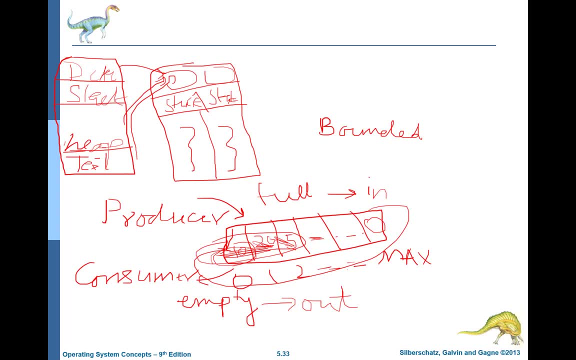 when the producer reaches this area again, it will start from here: the consumer. so we need to take care of these things. how many numbers are there which the producer has produced but the consumer has not consumed? maybe that the the producer has consumed but the consumer has not consumed. maybe that the 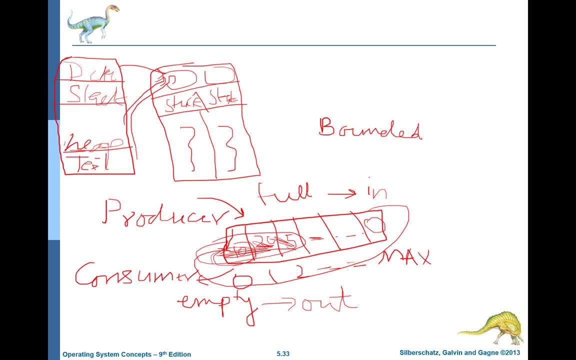 producer and cents and more are pointing to the same location, which means that the producer is going to produce next somewhere here and the consumer has received already. so that, how do we know this? for this we have another pointer, which is called counter, and the counter it contains the number of. 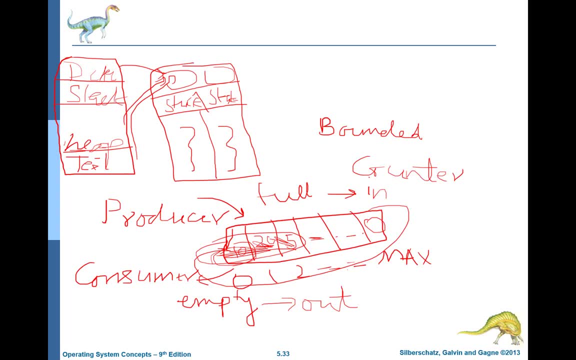 items available. okay, so how many items are there? if the counter is zero, it means that the consumer has consumed everything. if the counter is more than zero, it means the consumer can consume something more and the producer has produced something. now we need to care for these conditions, and that's what i'm going. 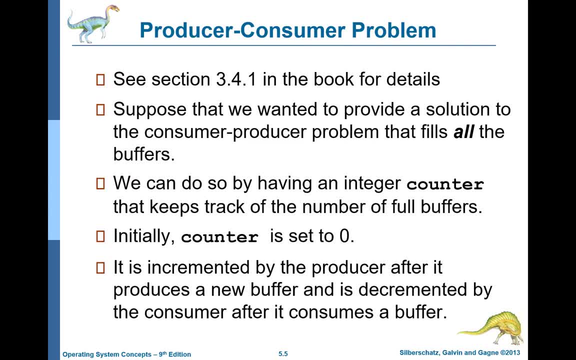 to now discuss in the slides. so suppose that we wanted to provide a solution to this consumer producing problem in which we fill all the buffers. okay, so the producer is filling the buffers and the consumer is actually, uh, consuming the buffers. okay, so we have an integer counter. 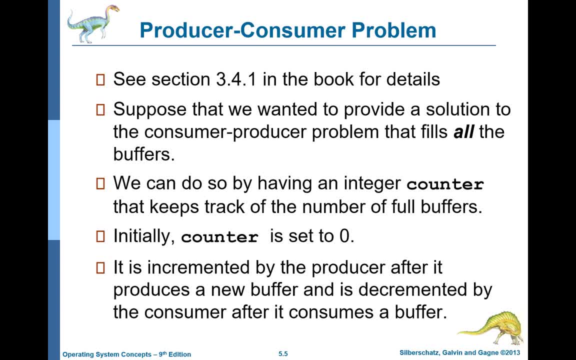 which keeps track of the number of full buffers- okay, how many items are available? and then initially we start when there is nothing produced by the producer. okay, so initially the counting is zero because every buffer is empty and, as the producer produces something, each time is incremented by one, and if the consumer consumes something, it is. 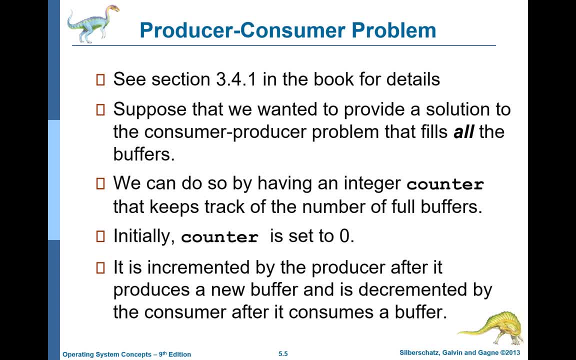 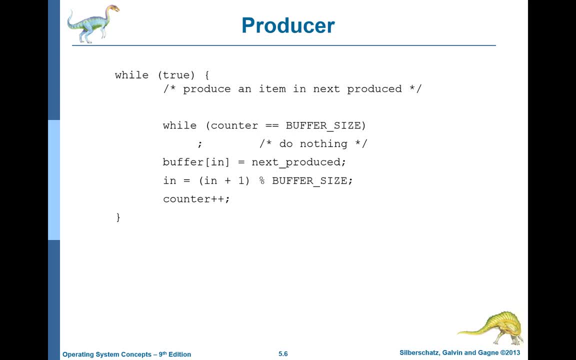 decremented by one. okay, so that's how we know how many things are there in the buffer. so the producer will use this code. what you can see in the first part, which says counter, is equal buffer. we want to check if the buffer is full or not. if the buffer is full, okay here. if this is true, the buffer is full and this: 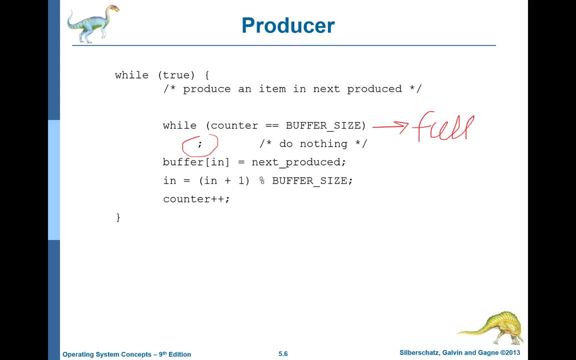 thing means after, while this thing means that actually it will be doing nothing. so if the buffer is full, the consumer, the counter is. Buffer size means the buffer is full because the buffer size may be 10 and the counter is 10, so the buffer is full in that case. 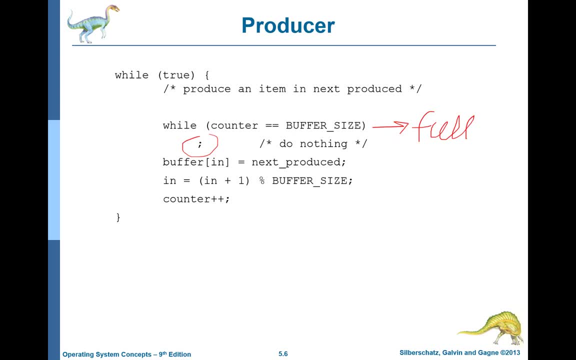 the producer will have to wait. so it will keep waiting. but if the condition is false, the buffer is not full- then Madam producer will go to this location, okay, which is the incoming bus base pointer, and it will produce something in this area. okay, that is actually the next item will. 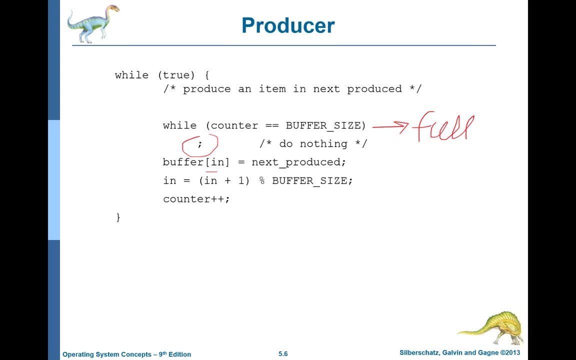 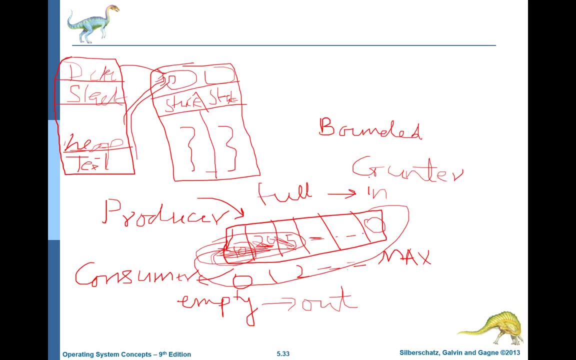 produce in this area and it will increment this pointer by one. remember i told you that if this buffer producer comes here, this space comes at the end here, okay, and this space is empty. so in that case, the producer will come again to the beginning, to the zero position. so how do we? 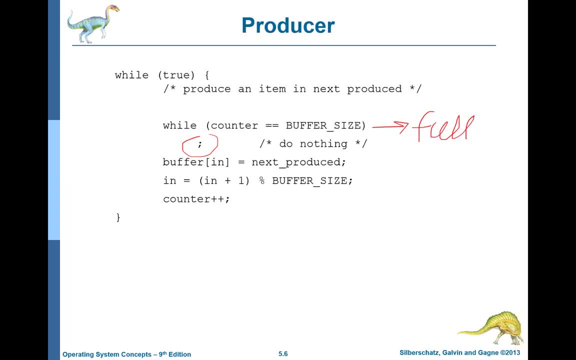 do this. we are using this statement, the model. can anyone tell me what is this percent sign and what does it mean? can anyone tell me? so if i say the value of n is 1, then and the buffer size is 10, then after this statement, what will be the value of n? 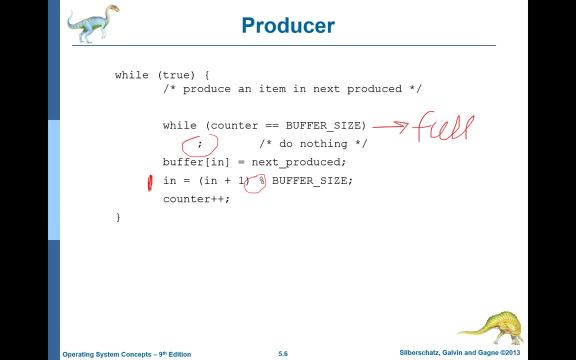 before it was one. now, when we execute this statement, what will be here? can anyone tell me? before it was one, and then i execute. so what is the value? this will become one percent ten. so what is one percent ten? what is ten percent ten? any idea? ten percent ten, this is equal to one, and one percent ten- sorry, ten percent ten, this is equal. 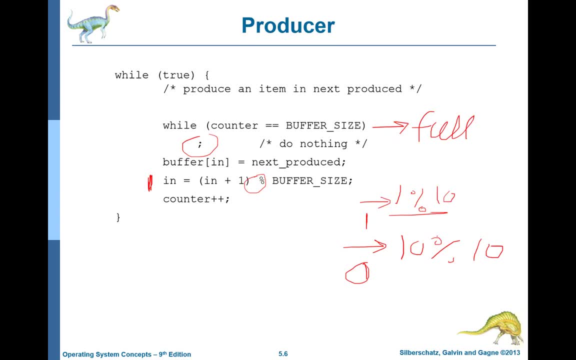 to zero and one percent ten, this is equal to one. okay, so the remainder, when you divide ten by ten, is zero, and then one divided by ten, the remainder will be one. okay, so when we execute this statement every time, it will give us the remainder divided by the. 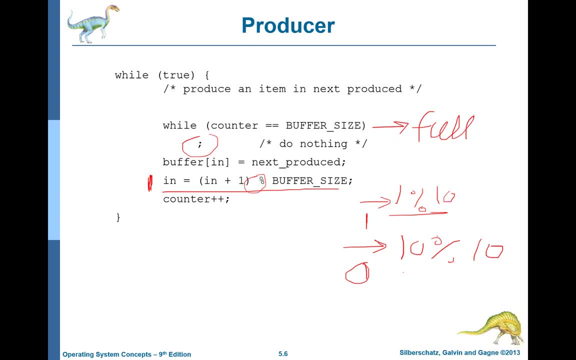 size of buffer. so if the size of buffer is full, okay, like in the condition, then the remainder will be zero. okay, it will start. uh, if the size of buffer is 10- and it was also at 10- then actually it will start from position 0 and it will start adding into the first position of the 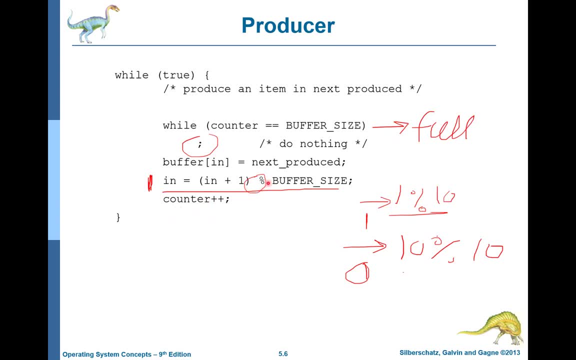 buffer okay, and every time we add something into the buffer we also increment the count. actually this is how we do. so let me repeat: first here, we check if the counter is equal to buffer size. let's say buffer size is ten and the counter is also ten, it means the buffer is full. it will. 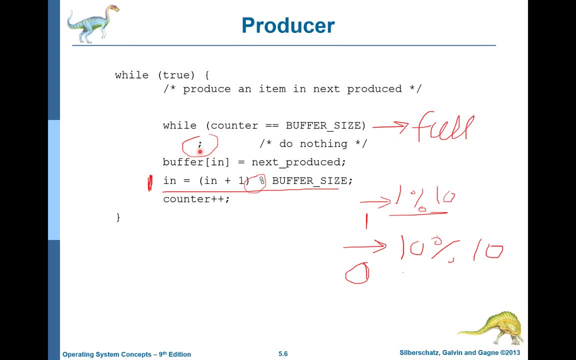 have to wait. it will not do anything in the while loop and this semicolon it means do nothing. but if this is false, then it will come here, it will produce something into this position which is in and which is 0.1 to the producing position of the producer, and after that it will. 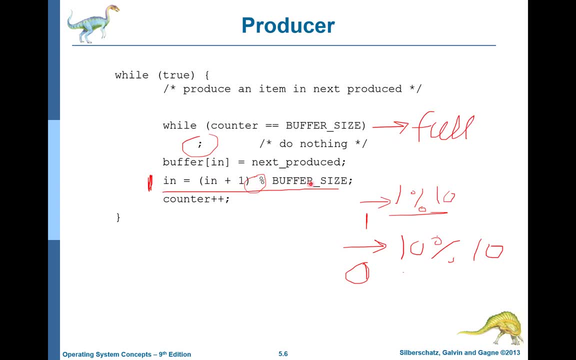 increment. now, here the important thing is, it will increment using this remainder. so if the new position comes to be the size of the buffer, it will start from 0. otherwise it will keep incrementing by 1. when they equal to the size of the buffer, it will always start from the 0 and the counter will also be. 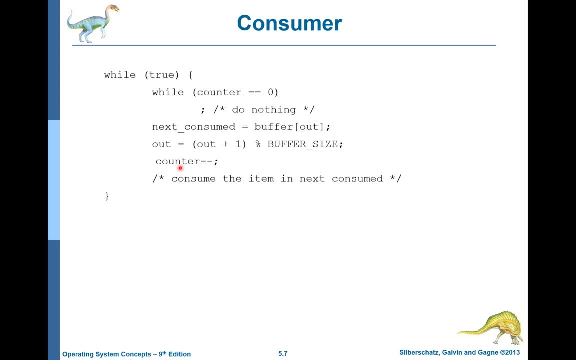 incremented because it has produced something. now we go to the code of consumer. okay, and it's similar to that of producer, except that the producer- here producer is checking for buffer size if it's full and the consumer is checking for empty. if the counter is 0, it means there is. 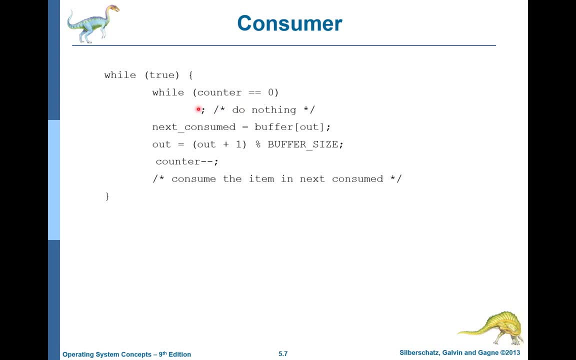 nothing to consume and it will keep waiting. similarly, if the counter becomes false, so it will come down and it will then consume something from the out position. the out position is reflecting actually from where this consumer will consume something. when it consumes something from this position, it will increment the counter of out by 1 and, just like producer, it will modulo. 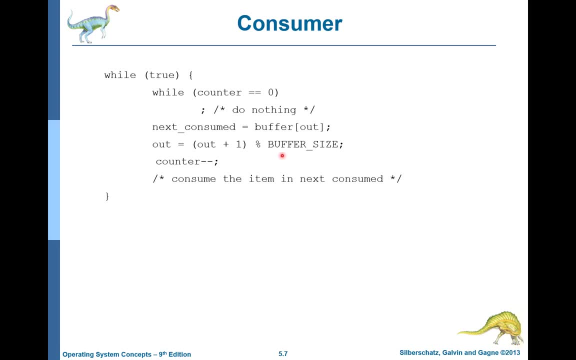 buffer size, which means that if it reaches the maximum size of the buffer size, then it will start from 0 again and it will decrement the counter, because it has conceived one thing. so the number of items, remaining items, or the number of buffers, is now one less. so this is how producer and 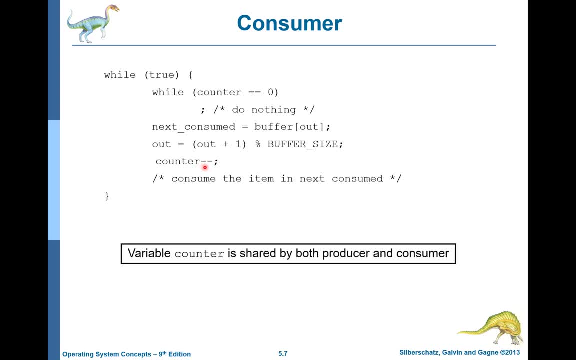 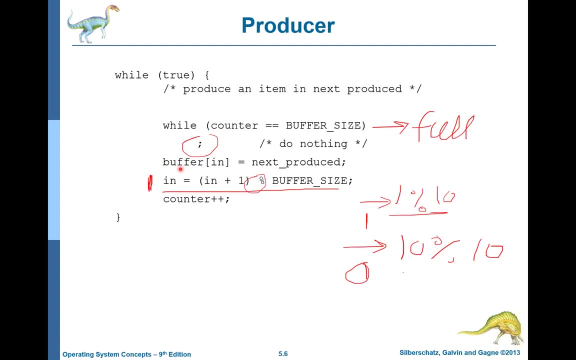 consumer. they both work. if you compare these codes, one is the buffer, which is shared, and the other one is the counter variable, which is shared between the consumer and the producer. so these two things are shared, but the change is being made in the counter variable. the buffer is just an array. wherever you want to make change in the array, it is. 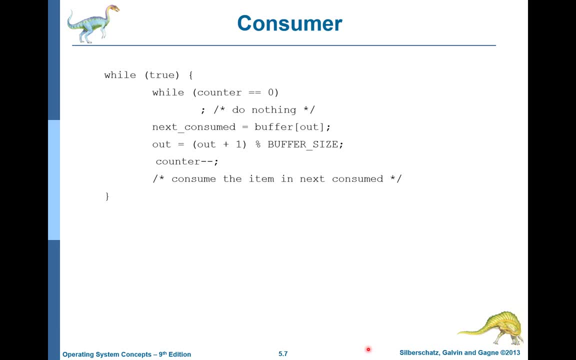 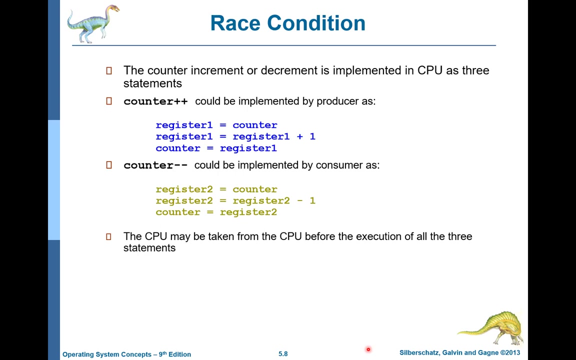 because of the counter. so we are interested in the counter because any change in the counter can be potentially a cause of error. so that's one thing. the second thing is that the counter can create an inconsistency, and that I am going to explain in the next slide. so I explained with the concept of race. 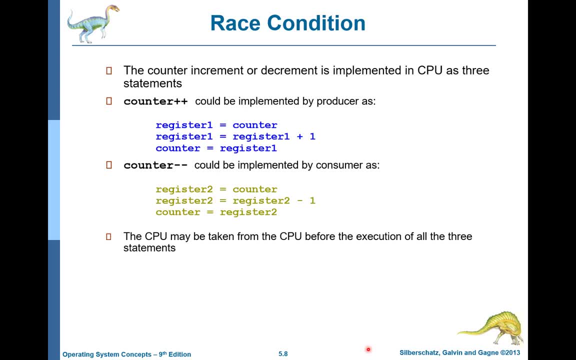 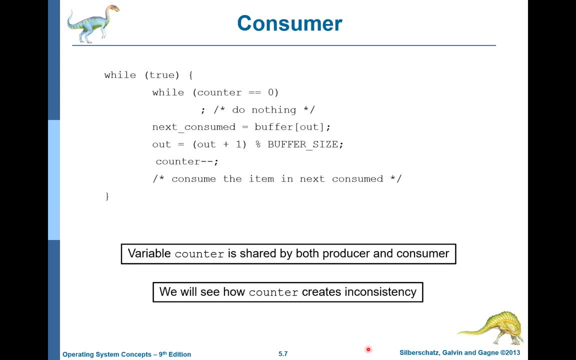 condition. ok, what is race condition? to understand the race condition first, let's understand that. the counter plus-plus or the counter minus-minus. what do you see? here is one statement in C language or in any programming language, but actually in CPU or in assembly language it is actually three. 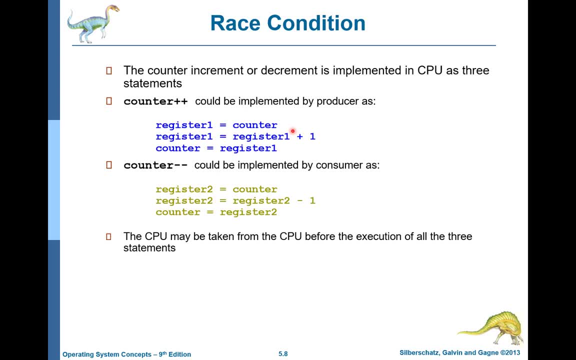 statements. why? because counter is a variable in the RAM. so in order to change something in the RAM, first you will actually bring the value of the counter to register, you will update the value of the register and then you will take the value of register to the RAM. you cannot change anything in the RAM. actually it's always. 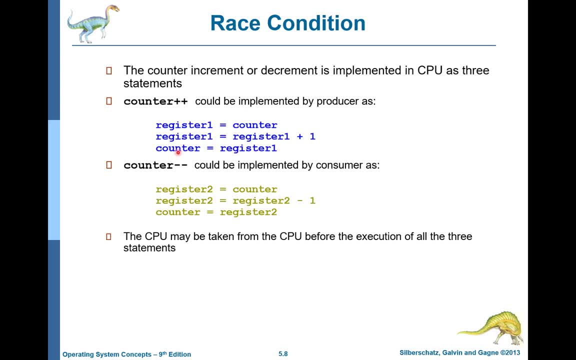 in the register that you change something in the CPU and then you copy the change from CPU to the RAM. so in order to update the counter, whether it's counter plus plus or counter minus minus- you have to bring the value of counter to the register- any register- and then you will make the change in the register. 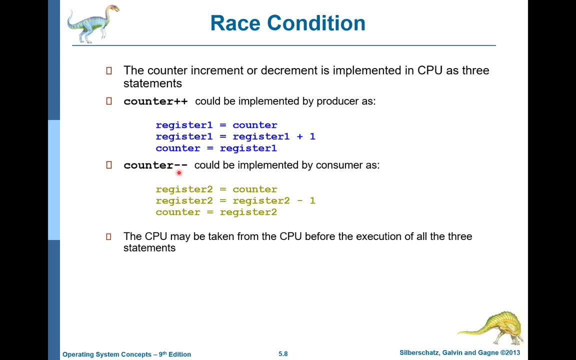 and send the updated value of the counter to the RAM in this way. there are three statements for incrementing the counter or decrementing the counter: okay, because in our case the producer is incrementing and the consumer is decrementing, so we have just shown two different registers. okay, they will not. 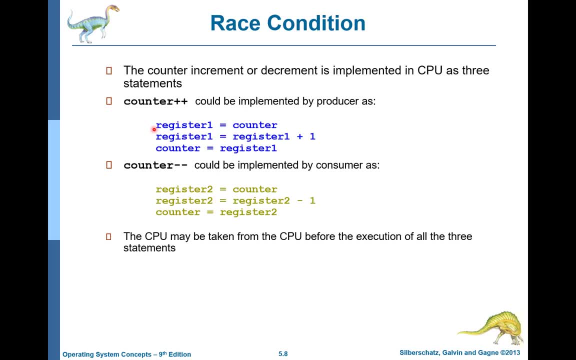 be actually working at the same time. why? because when producer is in the CPU it is using register, so consumer may be in the ready state or in the block state when the consumer, the producer, it leaves the CPU. so registers are updated by the value which are required by the. 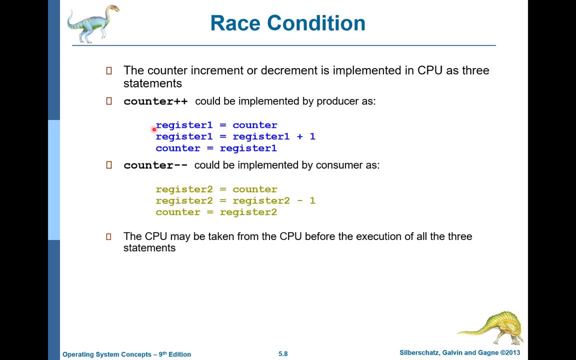 consumer and we have written register one and register two, but it can be the same registers because they are not used at the same time. okay, so it can happen that when the producer is in the register it is executing these statements and somewhere after statement one or after statement two, I mean before. 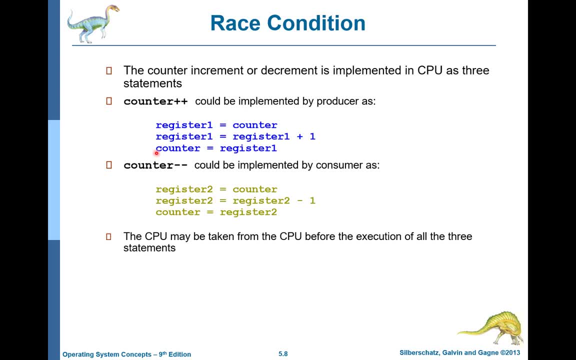 the completing of this third statement. we can stop this producer. okay, we can take the CPU from the producer and we can actually give registers to the consumer so the consumer process can come and it can continue. and in this way, in this way, maybe the register, the producer has not completed the execution. 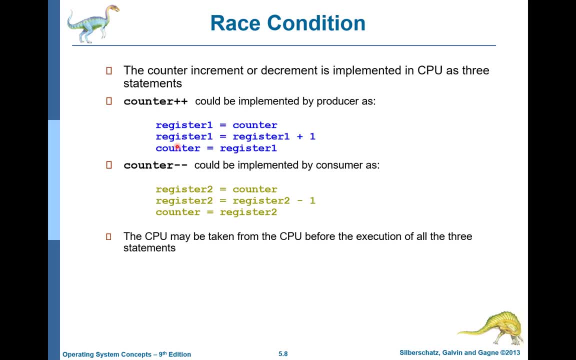 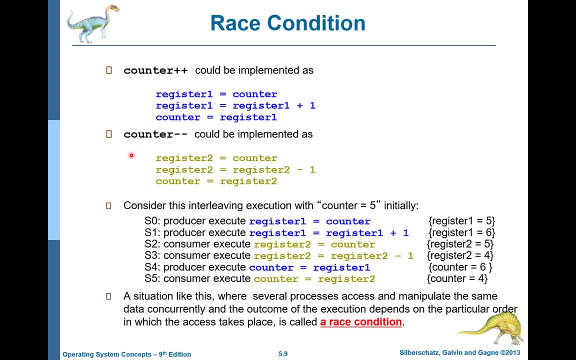 and consumer has come. so what will happen? there can be some problems. for example, let's say, consider these six statements from s0 to s6. what do you see here is that these six statements- three from producer and three from consumer- normally they should be this order: that the three statements of 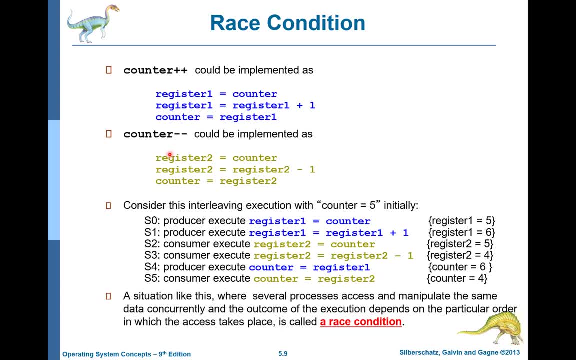 producers are executed first and then the three statements of the consumer are executed next. this is the desired way of execution but because of context, switch of process interleaving- and because the time lapse can expire for that process- for consumer or producer- we can switch the process in the middle of execution. So here is one example. 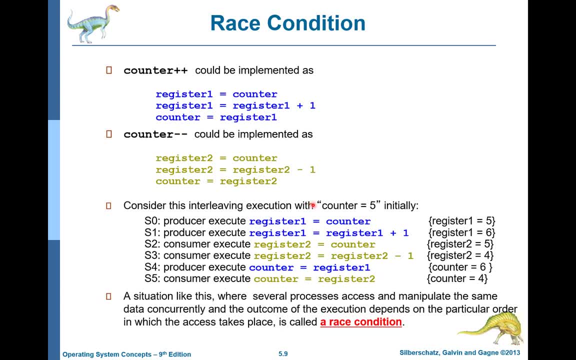 let us say, initially the value of counter was 5. ok, If we execute these 3, ok, then the counter of value will become 6, and then, if we execute these 3, the counter of value will become 5 again. So, after executing these 6 statements, in order, the counter value will: 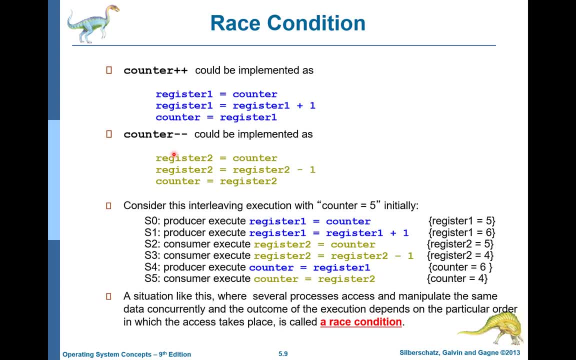 always remain 5. ok, that is the correct order. But let us assume the order is something like this: the producer it executes the 2 statements. ok, So the first statement is executed. the value of register 1 is 5 because counter is 5.. 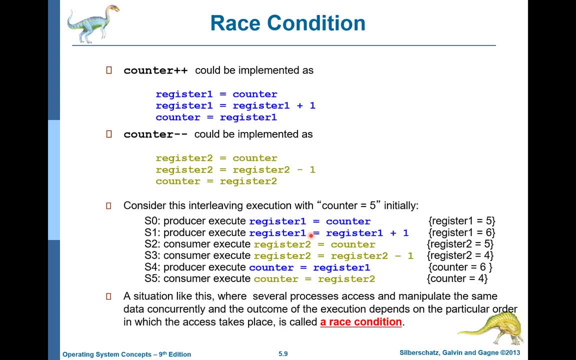 Then the second statement is executed. now the value of register 1 is 6, 5 plus 1 is 6. and suppose after that time the CPU is removed from the producer and it is the time of the consumer. Now consumer comes. it reads: the value of counter. the value of counter was: 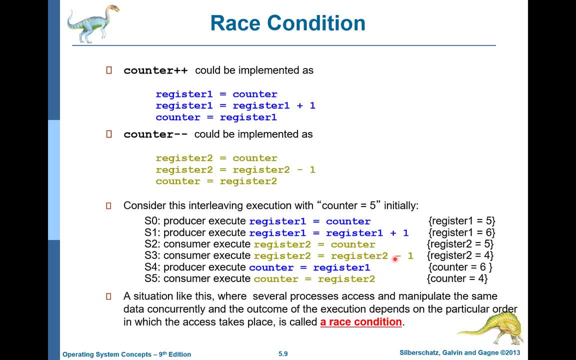 5. it updates the value of counter. now the value of counter is 4. ok, So what happens is That in register 2 the value was 4 and after that this process was removed from the CPU. the next instruction is execute. the next instruction that is executed is from producer. and now. 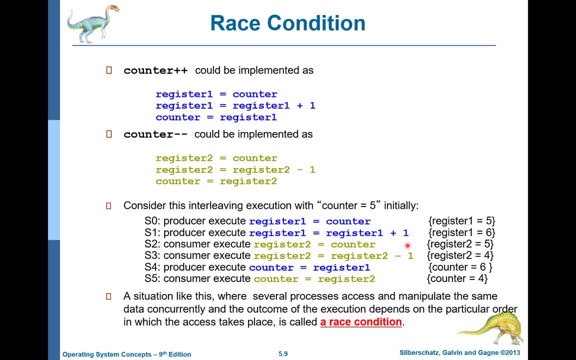 because before going the value of register 1 was 6. here again the value of 6 comes into register 1 and the counter becomes 6.. After this statement The CPU goes to register 1.. The consumer: when it comes, it reads the value from register 2. the value of register 2 was: 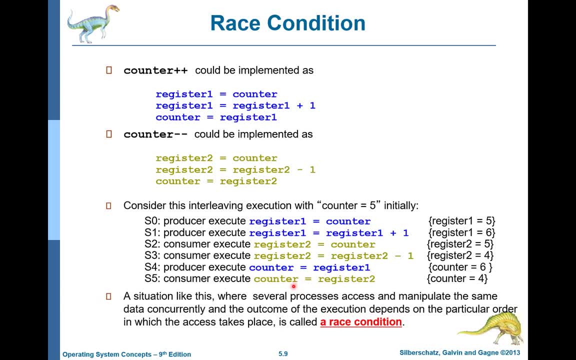 4, so the counter value becomes 4.. When this set of statements, it executes, it finishes. so at the end the value of counter is 4.. Actually it should have been 5, because it increments from 5 to 6 and increments from 6 to 5.. 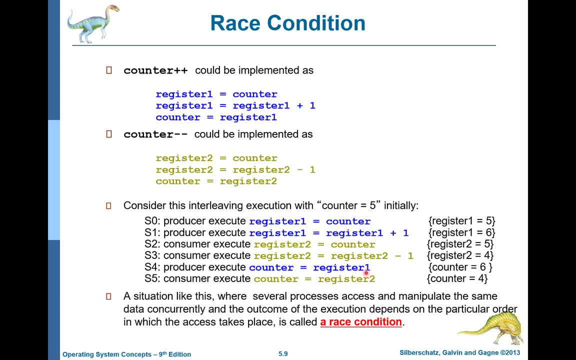 the end of these two executions the value should be 5, but because you see that here the value of the register gets 4, the counter gets 4 at the end. why? because these statements were not executed in the correct order, so this creates inconsistent data. that is called inconsistency of data. the data which was 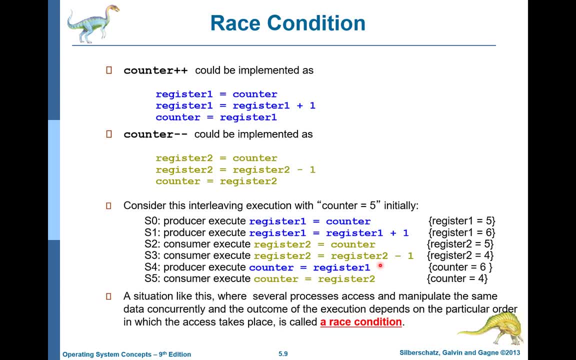 supposed to have the value of 5, the variable counter. it actually has the value of 4. similarly, you can rearrange these statements at the end you will see that the value of the counter will be 5. it is possible. or it can be 6. okay, it is. 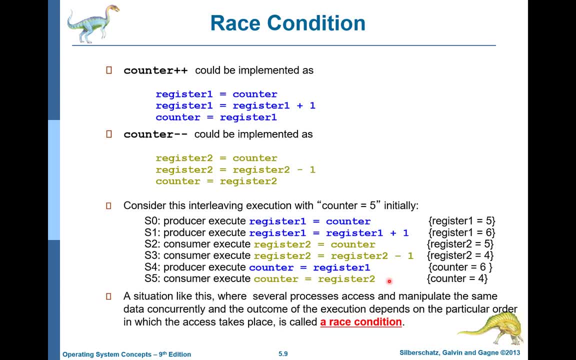 possible? it depends. so if you have this instruction before and you execute the instruction of register 1 after, if you swap s4 and s5, then the final value of the counter will be 6- okay, which is also incorrect. so this is a situation when two processes- okay, they are accessing the. 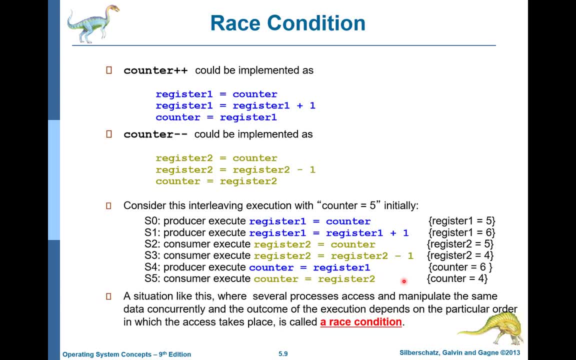 same variable counter at the same time, or actually in between their processing. so what you see here is that the outcome of their the execution will depend on the order of these instruction. it can be for the value of counter it can be 5 or it can be 6. 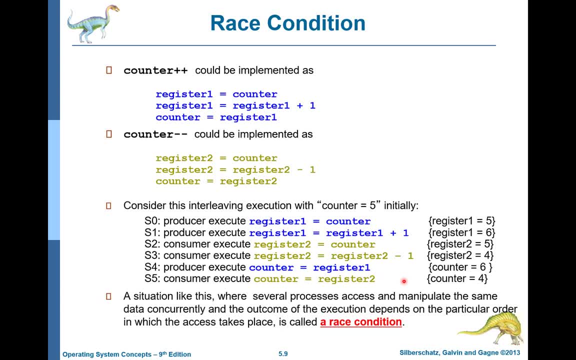 so, in particular, if you apply the initial expression with the fixer, check that, regardless of the order runner and runner bu, the full amount of functioning is controlled and your process comes to a regular state. yes, it, isayan, is at the low speed. well, the course that the students will face. 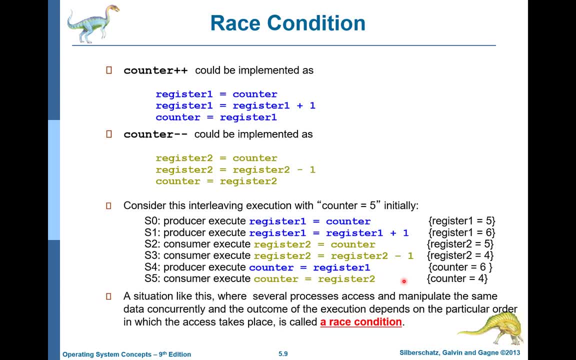 is at the low speed, if there is high speed expression of mobile operating condition, which can be and which can negatively affect the data. so how do we solve this problem? race condition: it can be solved if we give access to only one process at a time to access the shared variable. in this case, if this process 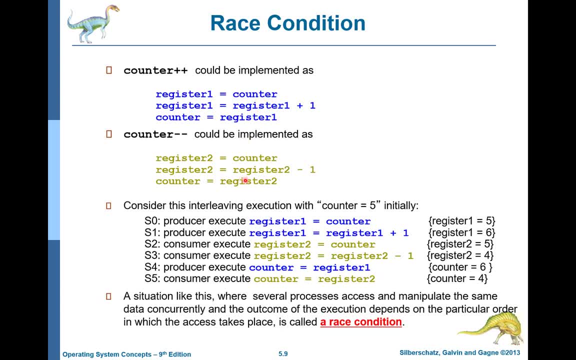 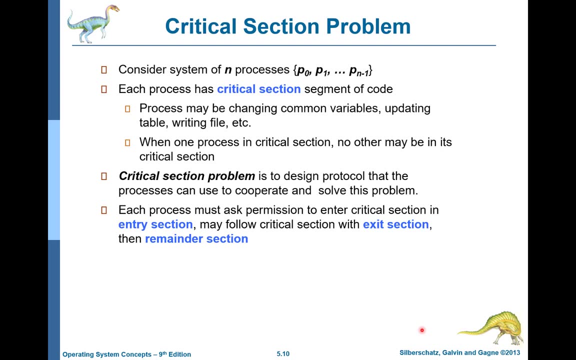 completes its execution before the consumer can come, then actually this consistency problem will be removed. so how do we do this? for this, we have something which we call a critical section. okay, so a critical section actually is part of the code in which the processes can have common variables. 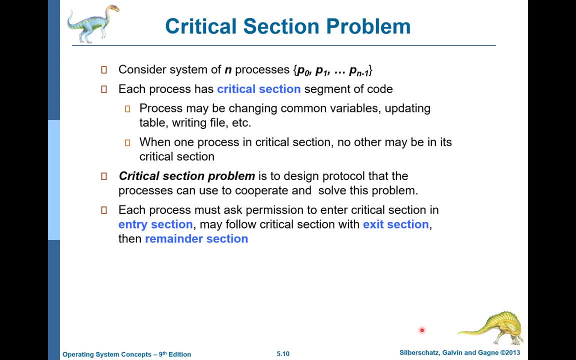 okay, and they can update or write or read these common variables at the same time or not at the same time, but actually it can be done at the same time. but actually it can be done at the same time. something which is shared between more than one processes, and it's possible. 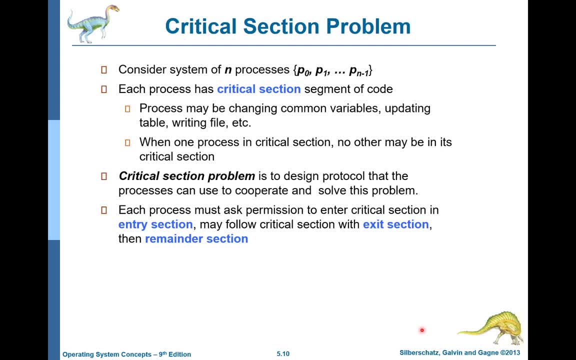 that every process, any process, can come and change the value of the variable that is called a critical section. okay, now here we can have two processes, or more than two process, any number of processes, the critical section problems. now the important thing is that if one process is in critical section, then 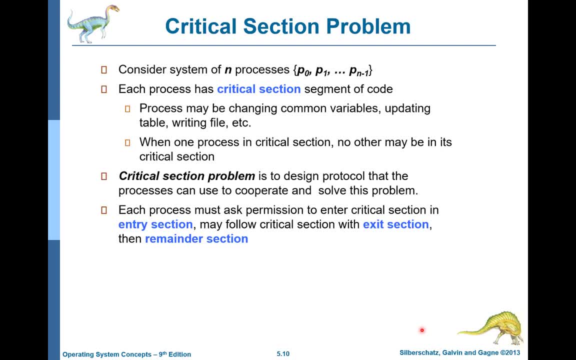 normally we should not allow any other process to come to the critical section, because if two processes make the changes at the same time, it can lead to data inconsistency. so the problem of critical section is to actually design a protocol that the processes can used to cooperate and solve this problem, which results in data. 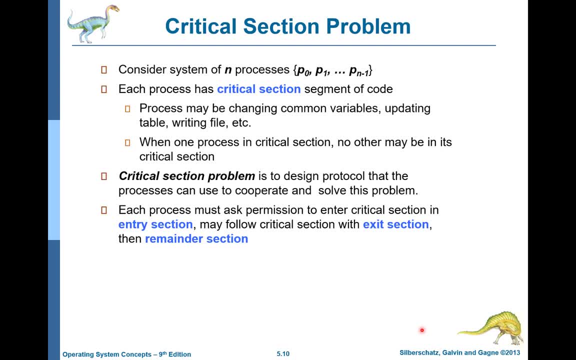 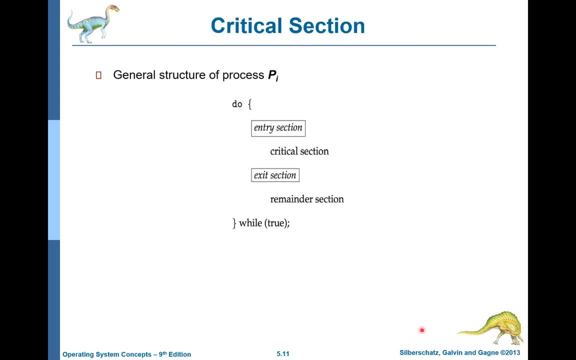 inconsistency. so how do we do this? for this we have actually the thing that the program code is divided into four different sections: the entry section, the critical section, the exit section and the remainder section. now, what do these four sections mean? the important thing, what we want is to protect the critical. 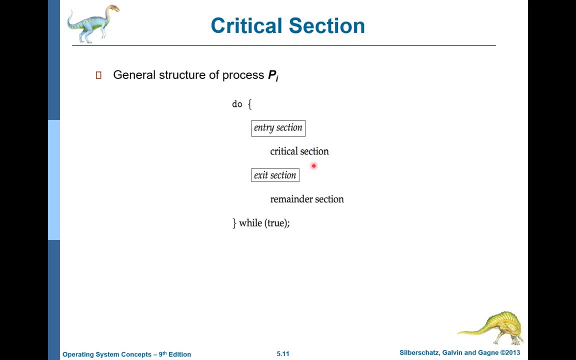 section from more than one processes to be entered inside. okay, so what you want is that before any process can enter into the critical section, it must pass through a entry section. Why? Because in the entry section, it will gain the permission to go inside the critical section. In this way, we know if there is any process inside critical section and, if there, 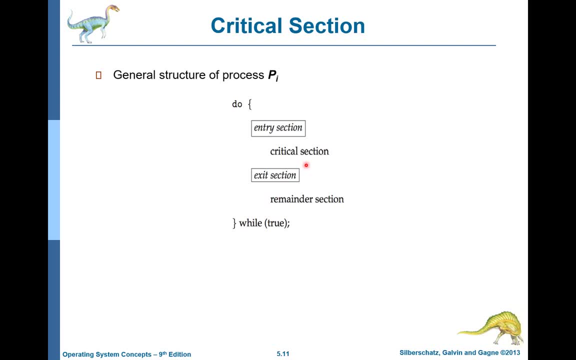 is any process inside critical section we may not allow other processes to go inside. So the other processes, they will be waiting in a queue at the entry section and when this process which is inside the critical section it leaves, it must go to exit section so that the other processes they know. 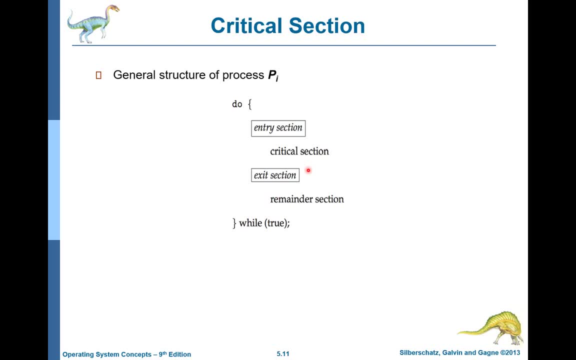 that the critical section is now available and they can enter. anyone can enter into this critical section. The remainder section is that section of the code which does not contain shared variables, so it can be any normal section and it does not have any negative effects or undesirable effects. 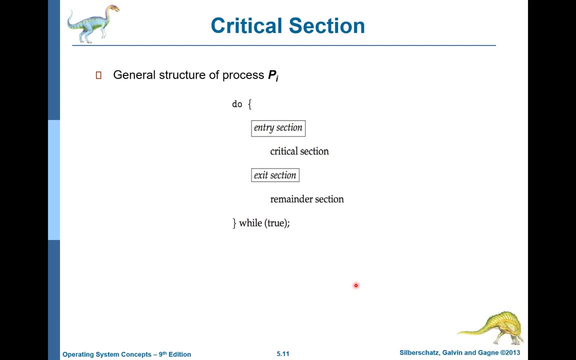 when the process executes in it. Why is entry section and exit section important? Let me give you an example of the real world. Let's say there is some room somewhere in your house or anywhere and this room is such that only one person is allowed to enter the room at a time. If any person is inside the room, no other person. 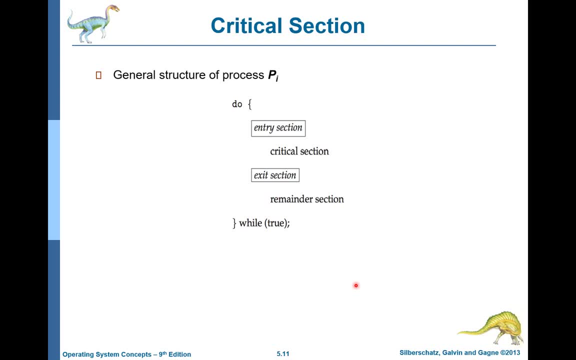 can go, and when the person comes out of the room, then the next person can go inside. So how can we design this problem in the real world? Can you think of a solution? How do you make sure that only one person can go into the room? So you may be thinking that, okay, we should. 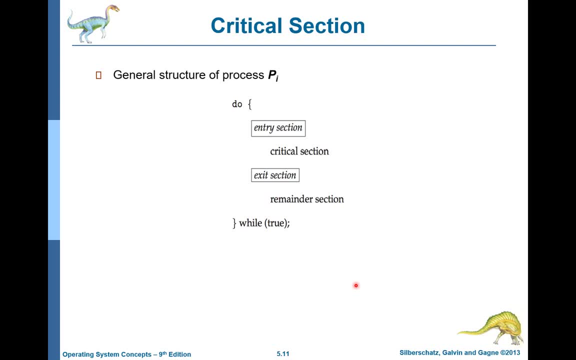 have someone who is waiting outside the door and when one person comes, they allow only one person. Yeah, that's one reason. Okay, so we can say that there is someone who is allowing one person, only one person, to enter inside, or we can say that for this room. 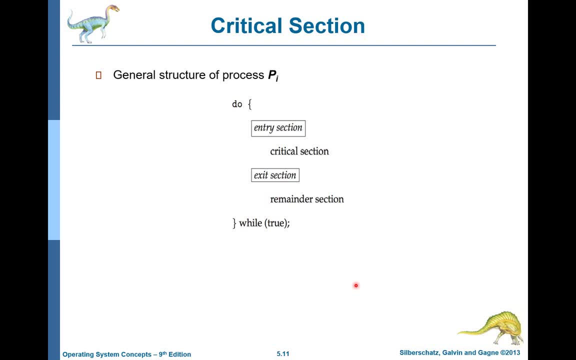 we can have a key and lock the room. so when a person goes inside the room, he or she may need the key. they will take the key from the entry section, they will go inside the room and then no one else will have the key to go inside. so they are waiting outside and the person who is inside 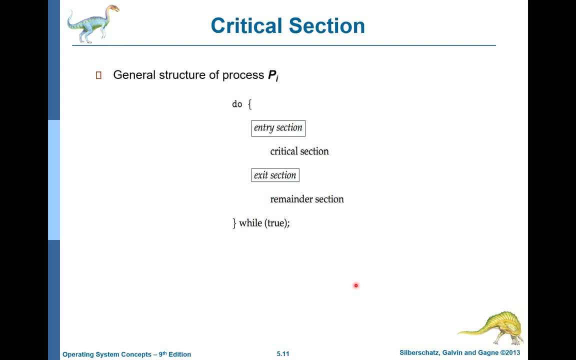 when that person comes out, he or she may give back the key. now, that is actually the exit section. the key can be taken by the next person and he or she can enter inside the room to complete their task. so this is the importance of entry section and exit section. okay, and just to explain this. 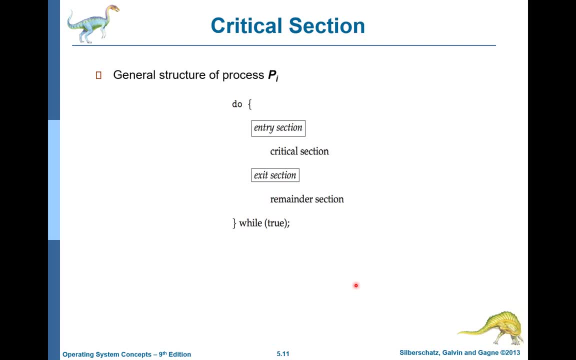 problem. we are using the while loop because a process may need to come again and again into the critical section, so we have this assume or a loop and here the remainder section. it can be doing anything else when it is outside the critical section. here it may not be editing. 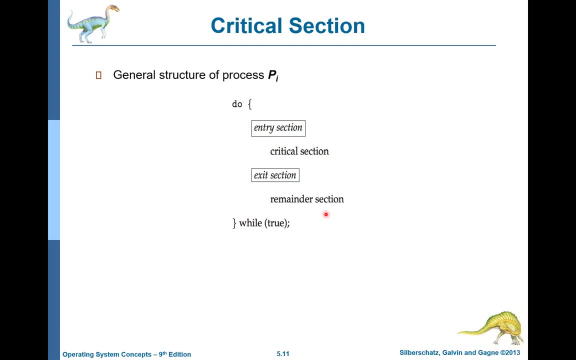 shared variables. okay, not updating or not changing shared variables, so there is no harm in executing this code by one process or more processes at the same time. so this small code and this blocks: they show the entry section and critical section and we are going to use these blocks to show the entry. 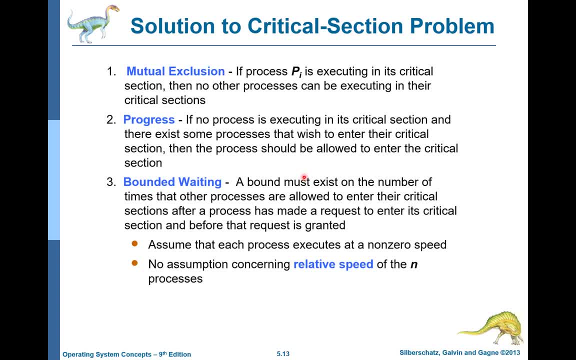 and exit sections in the actual algorithm. now for any solution to the critical section problem, the solution must be meeting these three requirements. the solution must be satisfying mutual exclusion, progress and bounded waiting criteria. what does that mean? mutual exclusion? in Arabic, we call it this, hasari, which means that 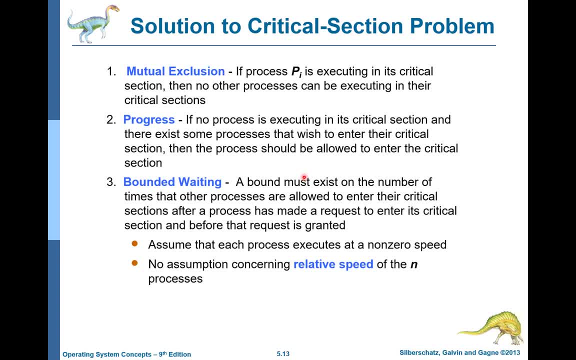 only one process is required to complete the entry section, so we are going to use this. one process can have access to critical section at the time, mutually exclusive. if any one process is inside the other processes, they cannot go inside the critical section. that's the first requirement. 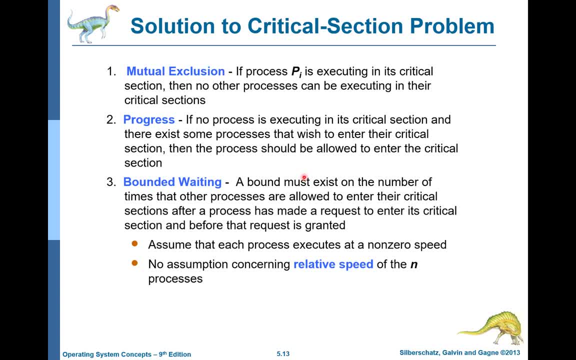 the second requirement is about making progress. okay, so let's say a process is outside critical section hardly goes right now into the critical section if the process is outside the critical section and the process does not need to go into the critical section right now, so it should not. 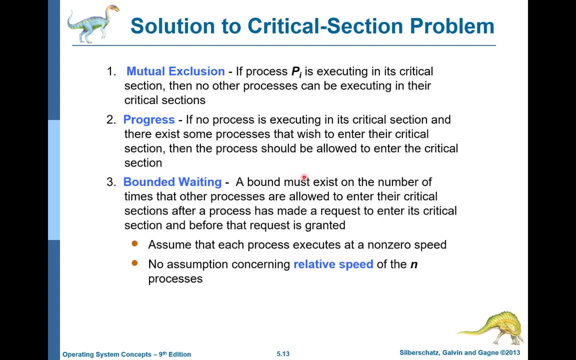 block other processes from going inside the critical section. and also, if a process is inside a critical section, it should make some progress and come out of critical section. so to make a progress, okay, to allow others to do the want, critical, sound progress- and come inside in critical section. you get to see our example and also work in the family- bounding, bounding, waiting. this is the third criteria. so there was another problem after this example. 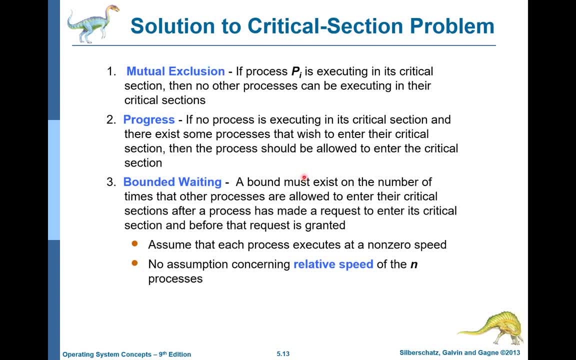 you are~ more problems later we do finally bounded waiting. 2. its general, the third criteria, gång. it says that the process must processes, but not must not wait indefinitely, okay, or for a very long time to enter into the critical section. what will happen is that, after some wait, this process 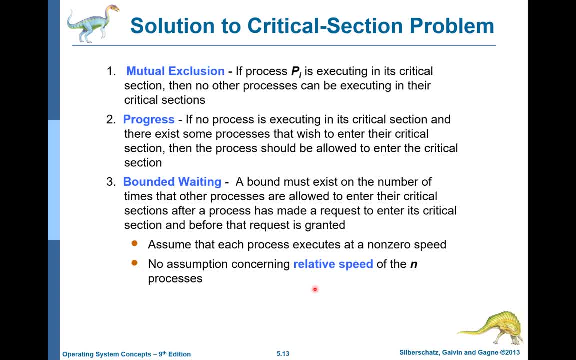 must be able to enter into the critical section and we have one assumption: that the process is executing at some non-zero speed, which means it is doing something, it is not blocked or it is not sleeping, etc. the second thing is that there is no assumption about the relative speed of and. 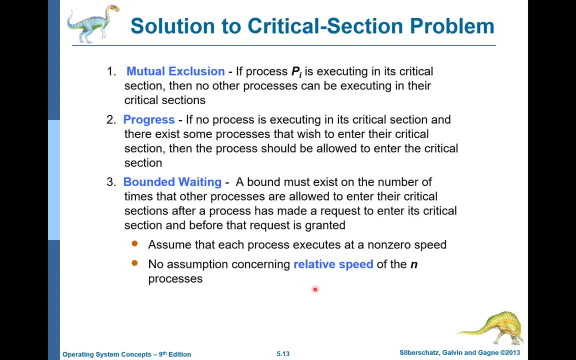 processes. one process can be very quick, the other process, it, cannot be so quick, so it's not important one is using cpu constantly or whether it is not using any cpu at all. okay, uh, it is time to break, but i think we will continue for a few. 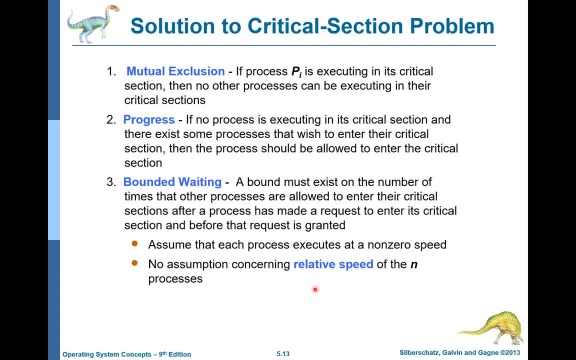 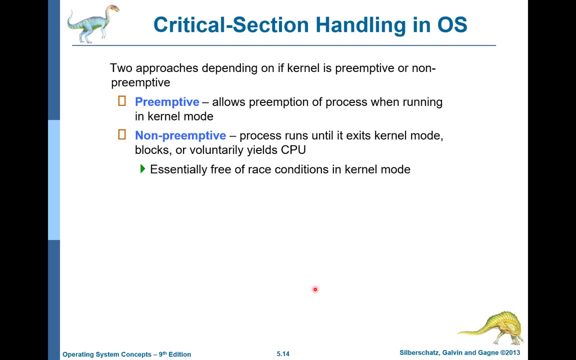 minutes and then for salah, we will take the break. so let's continue. understand these three conditions. they are very important, okay, usually i ask about them in the exam or in the quiz and you should understand what do these conditions mean? so in operating system we can also have this critical section problem. 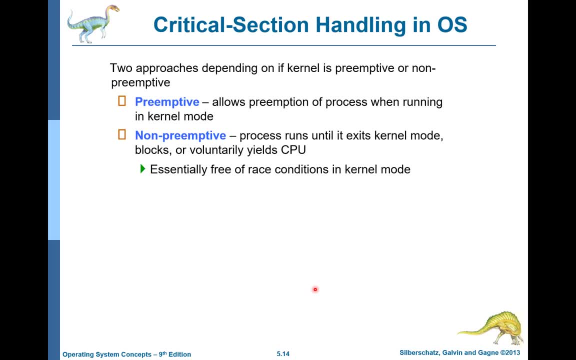 because you know, the main or the most important part of the operating system is the kernel. okay, so if a process is in kernel mode, okay, then how do we handle the critical section in that mode? okay, so we need to distinguish between two types of kernel design. one is the preemptive design, the 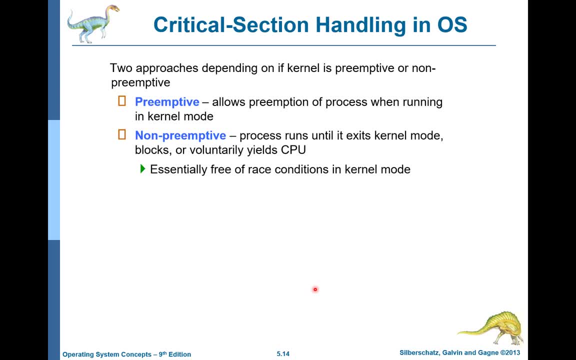 other one is the non-preemptive design. preemptive design means that if a process in kernel mode is running in the cpu and there is some interrupt, so this process can immediately leave the process in the cpu without finishing its task. that is preemptive. preemptive means you take the cpu from the process. 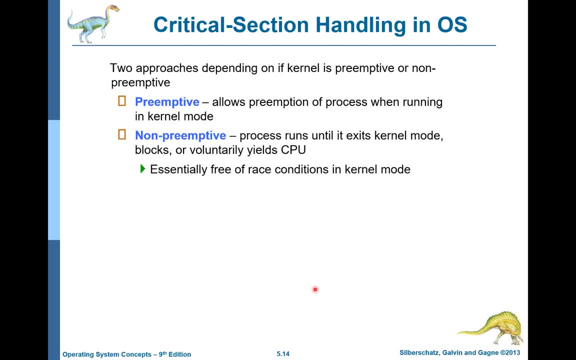 in non-preemptive. you don't allow an interrupt when a kernel mode process is executing in the cpu. so it means that once a kernel node process is in cpu and it is non-preemptive kernel process, so it will complete it, its task. if there is any interrupt, trap signal, whatever, it will continue to completing to. 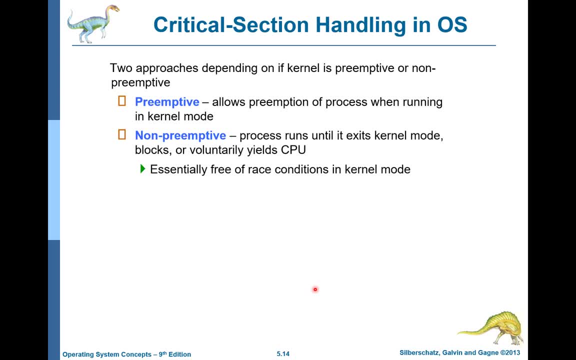 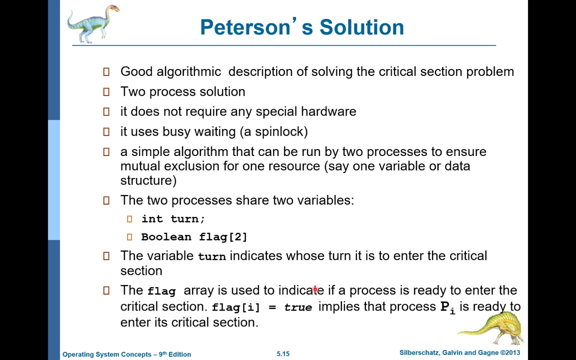 complete its task and when its task complete then it will leave the cpu. so these two processes, type of design- are important in when you design a kernel- okay, and it plays a role in how fast or how responsive is an operating system. so what are the solutions for solving critical section problem in this course or in this chapter? 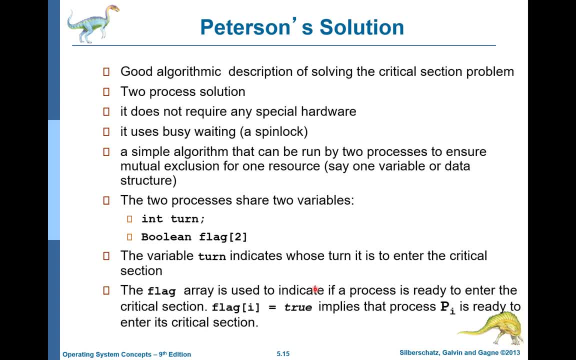 we are discussing three types of solution for solving critical section problem. the first one is the peterson solution. peterson was a person who actually designed the solution for critical section, so this solution has one problem limitation: that it works only for two processes. in reality may be there are a hundred processes which want to access the critical section. 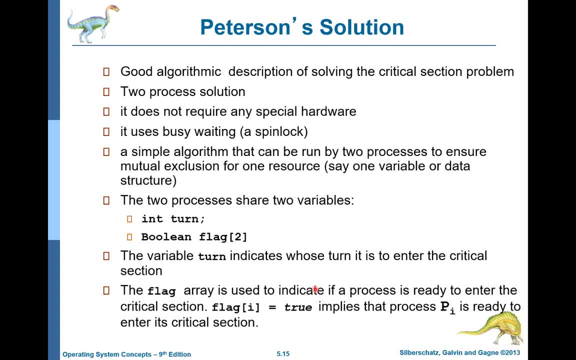 so this is not a very scalable solution. it can work for two solutions, but it is elegant because it does not use any special hardware. it can be just done using normal software instructions. okay, so the concept is that two processes, they share two variables. one variable is a process and the other is not a process. 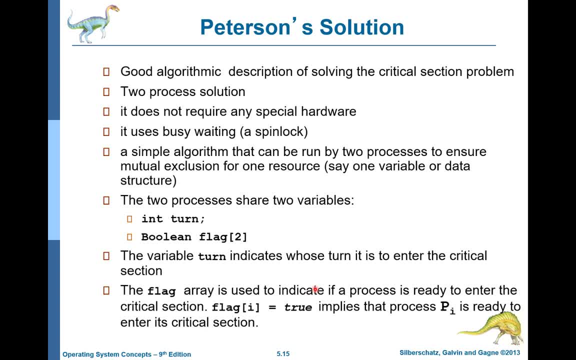 so the concept is that two processes. they share two variables. one variable is the starter process and the other is normal version, meaning 2 products, par test cells, and if you Bloom, two is a struggle term. the other variable is flag. turn is type integer. flag is an array of type boolean, because 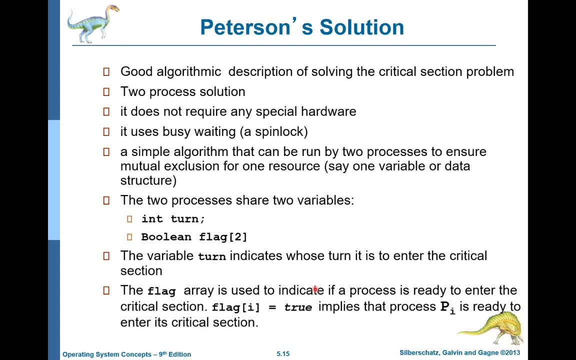 we are dealing with two processes. so the flag has two positions: position zero and position one. let's say the process one is process zero, actually, and the other process is process one. so at position zero we have information as true or false about process zero and at flag, position one. 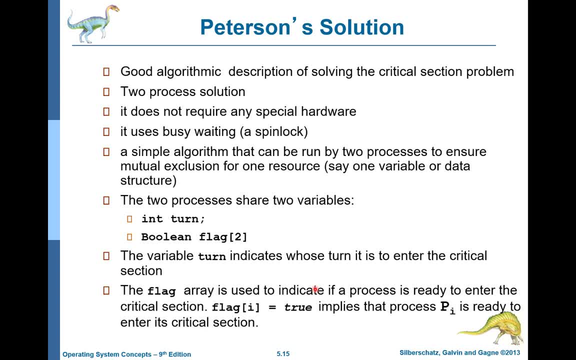 we have information about process one, the variable turn, which is an integer. it indicates whose turn it is to enter the critical section, whether it's process p0 or p1 which is going to enter into the critical section, and the flag array is used to indicate if a process is ready to enter the critical section or not, whether the process wants to. 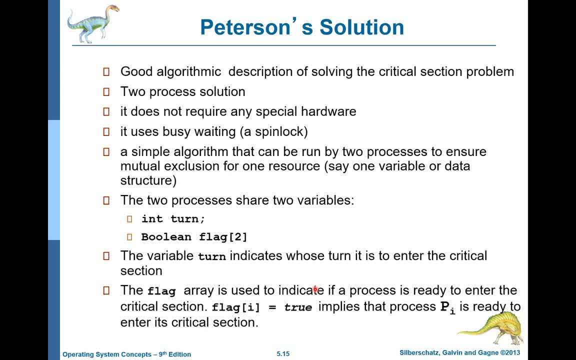 enter a critical section. so if flag 0 is true, it means process 0 wants to enter the critical section. if, like 0 is false, it means process 0 is because false. it does not want to enter the critical section and in that case the other process can go inside the critical section. 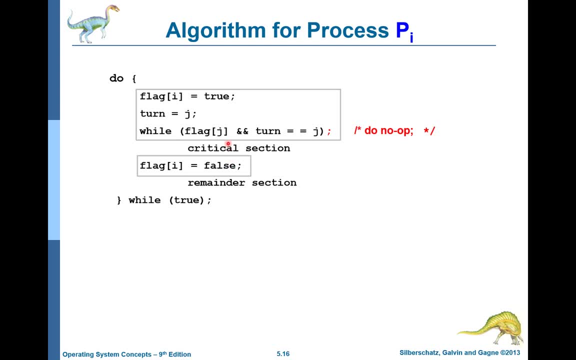 so this is the code in the boxes. you can see the entry section. so this is the entry section and here is the exit section and in between these two there is the critical section. so in entry section, if there is no other process in the critical section, this: 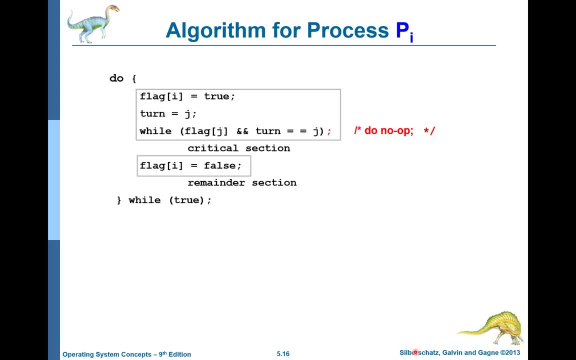 process will immediately go to the critical section, but if someone is already some process is already in the critical section- then it will keep waiting. how? because we can see it is using this while loop and it is not doing anything but just busy waiting. this is called busy. 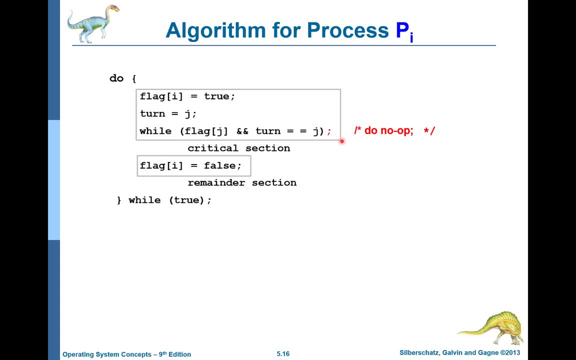 waiting. actually it is waiting, but at the same time it is busy for checking the while condition continuously. this is actually the algorithm for process pi, so we can assume one process is pi, the other process is pj, so this code is executed by process i. here flag i is equal to true, which means 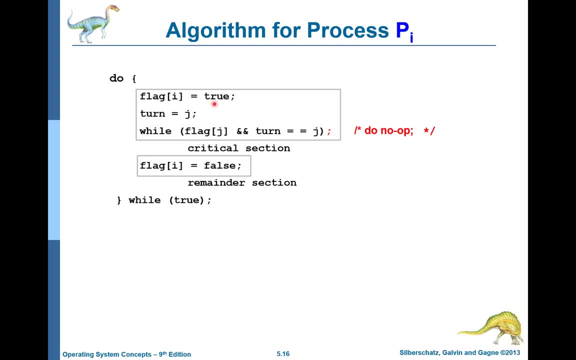 that this process wants the term to be true, it wants to go into the critical section and we say that right now the other process in the critical section. okay, we assume, let's say, they are in the critical section so we cannot go directly inside, but we will check if it's available or not. for 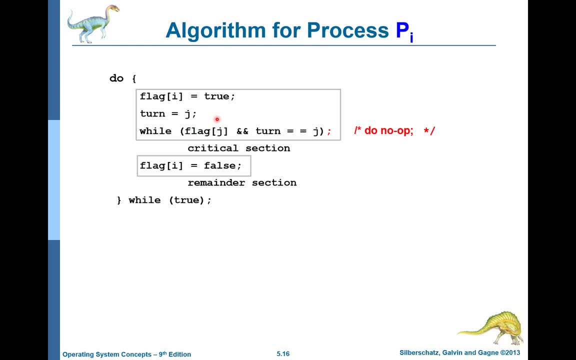 that again we have this while loop and inside while loop you have two conditions. now before, in the previous while loop, if you remember, there was one condition okay, and here we have two conditions. which says that while flag is j, which means the other process is interested, and turn is 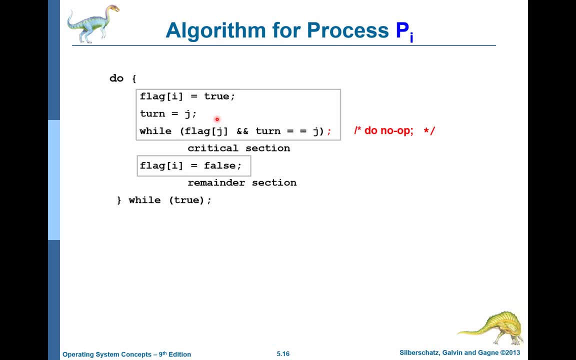 equal to j, which means the other process is: this is the turn of the other process, because he is inside, so it will keep in the loop. now, you, you, if any of these is false, flag j becomes false, which means the j process is not interested, so it will violate the condition and this while loop will be false. or if the turn is not j, if turn is: 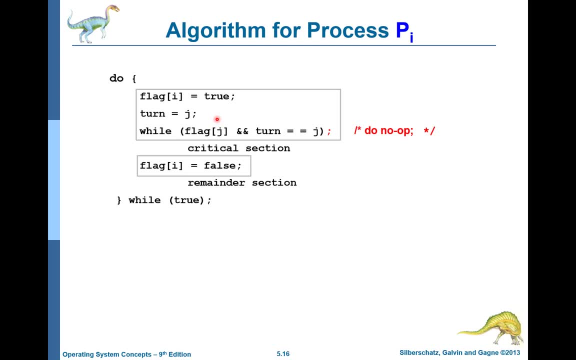 not equal to j, it is some other number. for example, turn is equal to i, etc. then it means that turn is false, which means that the other process, j, is not inside and process i can go inside. okay, after any of these conditions falls, then you can enter the critical section and when you turn, 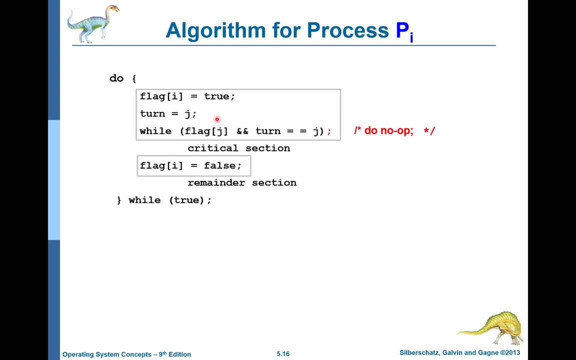 out of the critical section. when you get out, you will make sure that your own flag is false to show the other forces that you are not interested, and you can then go to the remainder section. now the problem with this peterson solution is that it works on alternating basis. 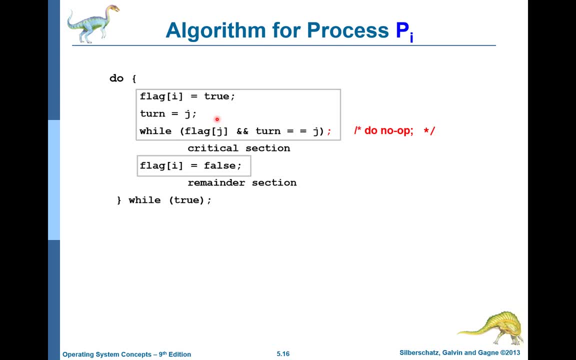 which means that when process i comes out, then process j can go, and when process j comes out, then it has to wait for process i to go inside and come out. so any process cannot go two times or more than two times in the same critical section. it is based on alternating entrance. if i is gone inside and come outside, then j can go inside and come outside, and if j has come outside, only then j has to wait for process i to go inside and come out. so any process cannot go two times or more than two times in the same critical section. it is based on alternating entrance. if i is gone inside and come outside, then j can go inside and come outside, and if j has come outside, only then j has to wait for process i to go inside and come out. so any process cannot go two times or more than two times in the same critical section. it is based on alternating entrance. if i is gone inside and come outside, then j can go inside and come outside, and if j has come outside, only then j has to wait for process i to go inside and come outside, and if j has come outside, then j. 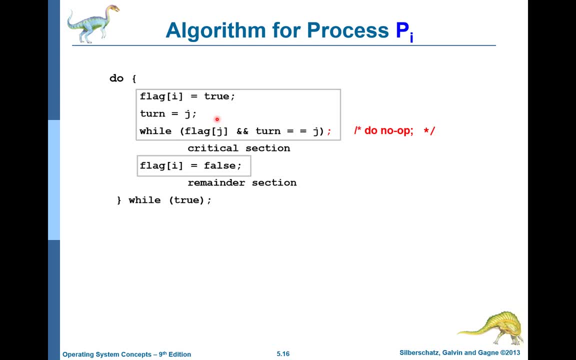 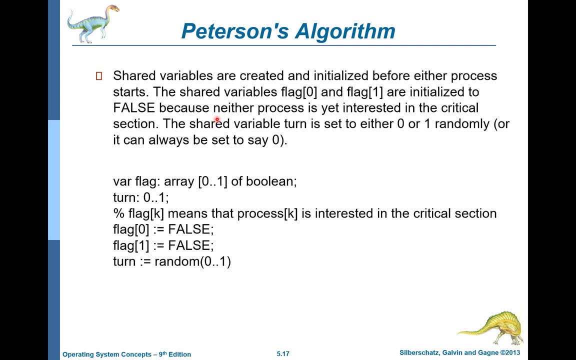 then i can go inside. so this creates a problem. this algorithm is described here on this slide. okay, the detail is here that you have a variable flag which is an array of two indices, one for one process, the other one for other. this is a boolean array. turn can be zero or one. so for process p i, if turn i is zero. if turn is zero, okay, then it means 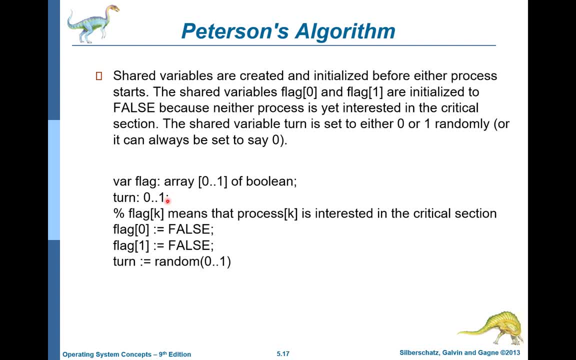 that it is this process term. otherwise it will be the term of the other process. okay. similarly, flag false: it means that this process is not interested. this flag is true that this process is interested and we can decide in the beginning if it's term. randomly choose zero or one to decide. 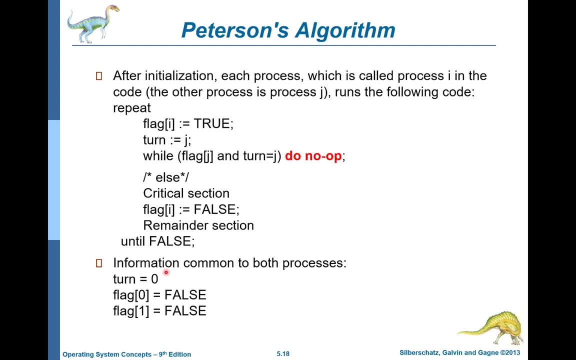 which process will start. it can be any process which starts, so that was about the initialization. after this, we are in a loop, okay, and in this loop, what you see is that you check for flag j and the turn of the process. if they are false, okay, then you can enter the critical section. 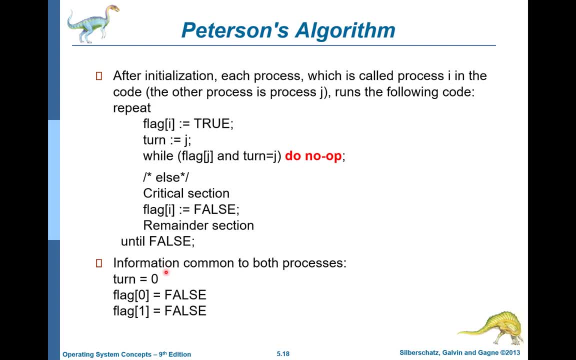 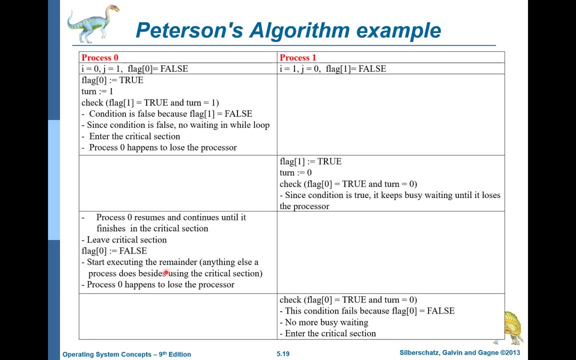 and change the flag and you can go into the remainder section. so this is about actually peterson's algorithm. now, this example i could have explained, but i don't want to explain to you. i want you to please study it yourself. okay, how does it work? okay, and if you have any problem, then you can ask me about this example. 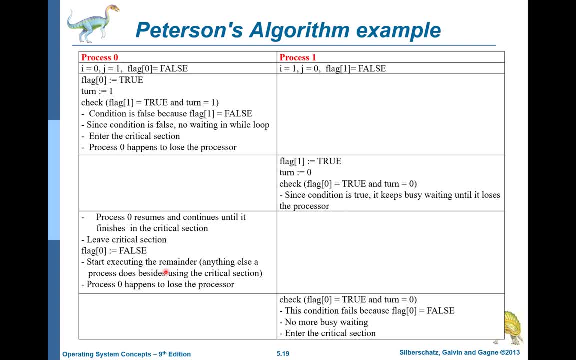 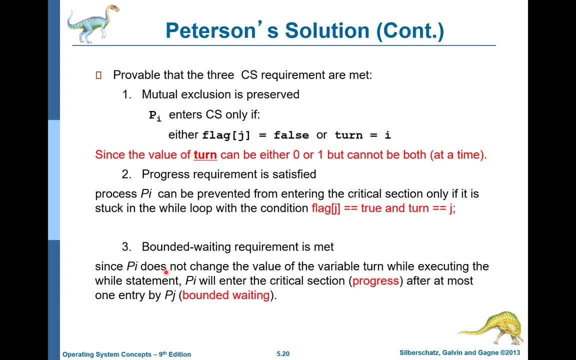 in the next class. briefly, it is showing you two processes, process p0 and p1, and what happens when they both, let's say, want to access the same critical section. so this is the example now, as we discussed before, that for every solution, any solution to critical section problem, we must meet three. 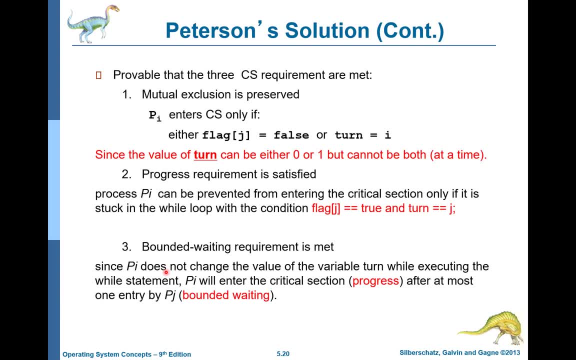 conditions. number first condition is mutual exclusion, and we can see that this peter says solutions. it can preserve mutual solution. why? because a process can enter critical section only if flag j is false or turn is i, and because the term can be either zero or one, which means that it can be either belonging to this process or other process. so this way, 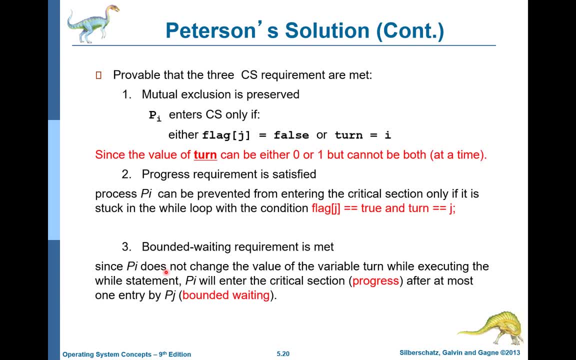 it can be accessed by any process, only once to enter and then they will change the value, so it is turn by turn possible. the second requirement is that about progress. okay, and the reason is we make process because this condition can be true or false when the other process actually finishes and it sets the value of flag to the other process. 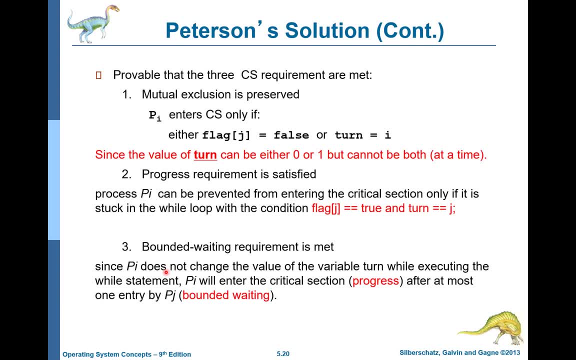 in the exit section, then it is actually as form of process progress. the third one is bounded weighting requirement, because it is making a progress and because every process is alternating here. so process p0, then p1, then p0, then p1. in this way there is 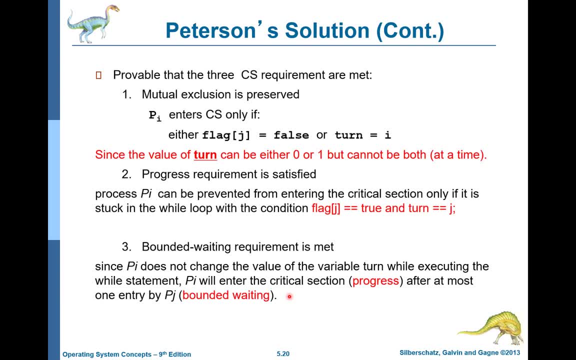 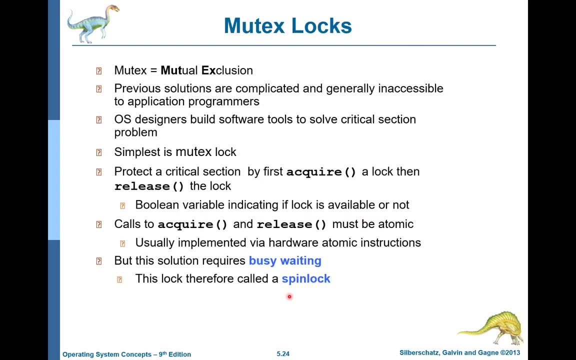 just bounded weighting, the any process does not have to wait for a long time or for indefinite period. so that was the whole discussion about peterson's solution. okay, the second type of the second solution to synchronization problem between two of our processes is the mutex locks. what is a muted mutex lock? mutex is a word which is a combination of mutual and exclusion. 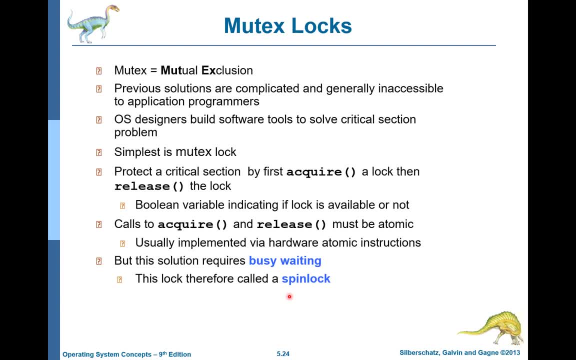 and in the previous slides i explained to you what is meant by mutual exclusion. okay, so mutex means mutual exclusion. okay, and what we have is that mutual exclusion lock requires support from hardware. okay, this needs some special hardware which can execute atomic functions, which means only one instruction at a time. okay, so here you can see that you have two. 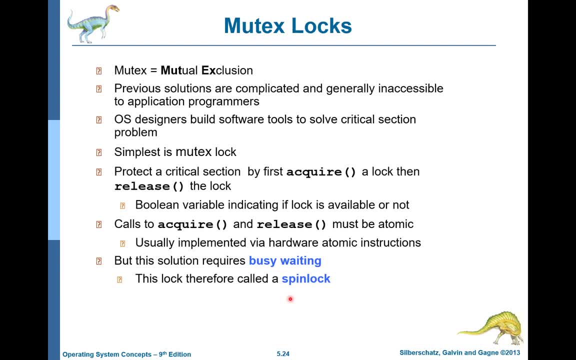 methods. one is called acquire and the other one is called release. before i gave you the example of key. if you want to enter a room, if you have a key, you can enter and once you finish you come out, you lock the room and give the key to someone else. this is the same here. 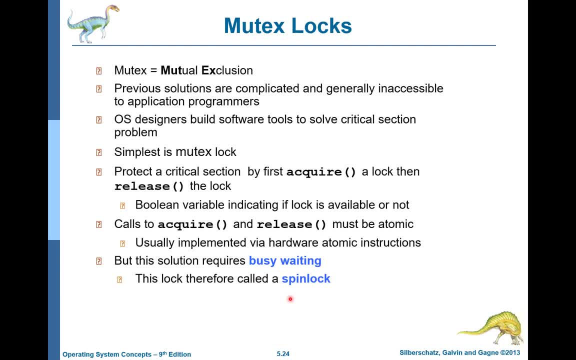 we can assume a key and someone who has, who calls the acquire it's cross. it needs the key and when it gets the key, then after finishing from critical section, it releases the key using the release statement. okay, so, as i told you before, the acquire and release, they must be atomic, which 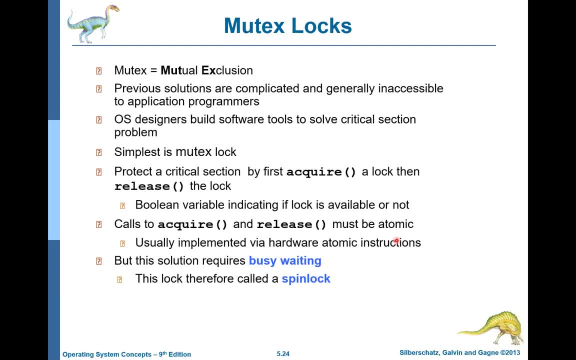 means that they can be executed as a single instruction or in a single cycle. so that's why we have this solution and this is the solution of the process on the cpu. so this solution is busy waiting, just like the previous one, which means that there is a loop. 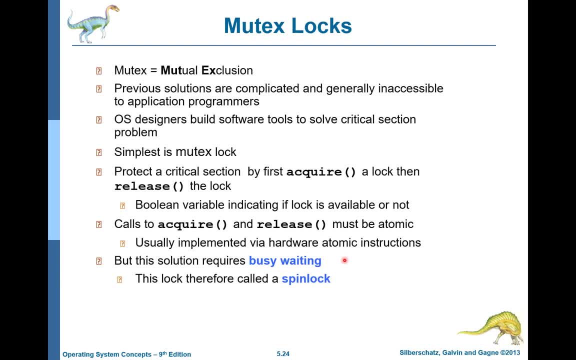 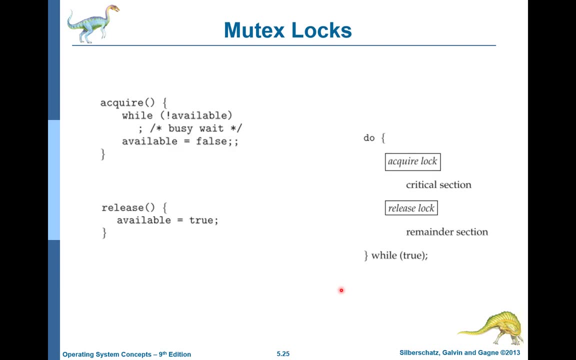 in which the process is busy but actually doing nothing. it is busy in what? it is busy in checking the condition of the variable okay in a while loop, and that's why this log is also called a spin log. a spin log means that you are waiting for this lock. 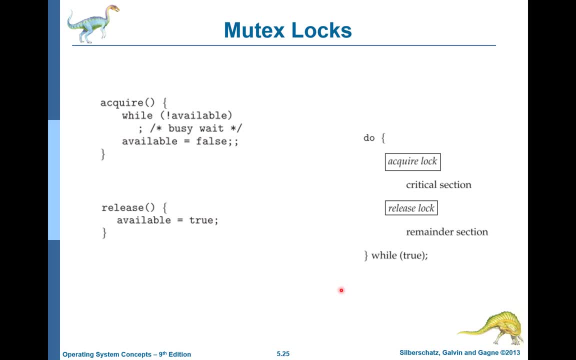 again and again. so these are two methods: one is acquired, the other one is release. okay, in acquire method, what you do is that if something is not available- let's say if it's not available, which we call the key, the key is not available, then it will not do anything. okay, this. 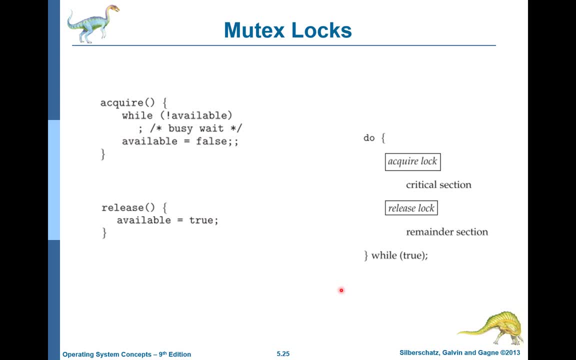 is called busy wait. it will check again and again while not available, so it is busy waiting, but once the lock is available, it it is true. so this condition is false and immediately after that, this process will make the available to be false. okay, so this acquire is actually working as. 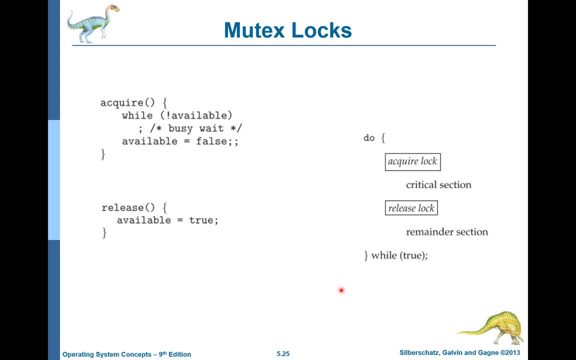 atomic: okay, and when someone is required, no other process can be executed in the acquire- okay. so after it comes here it says: available is equal to false. for all other processes this is false and they will be in the while loop. so after requiring the log, this process will go into the critical section and when it comes off the critical section it will. 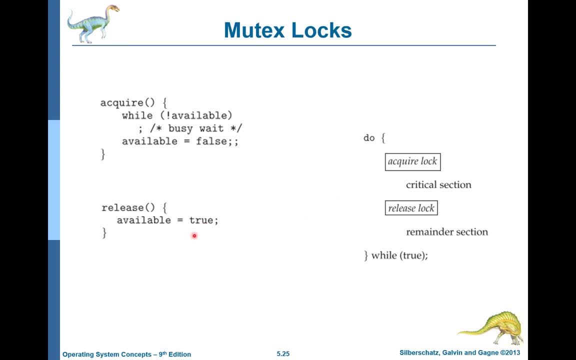 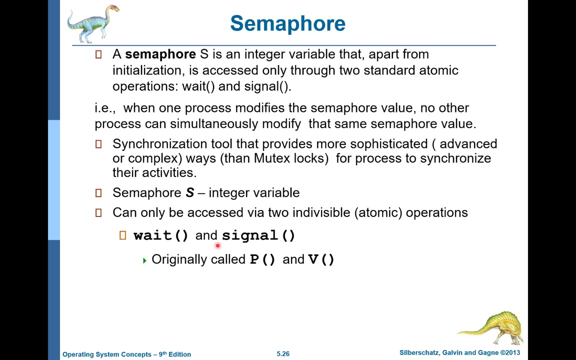 release the lock and for that it will make the available true, which means other processes can actually access this lock. okay, so let's take a short break. so we start again after the break. before the break, we studied about mutex locks. okay, inshallah, this chapter today. this is a small chapter, so after the mutex lock lock, the last. 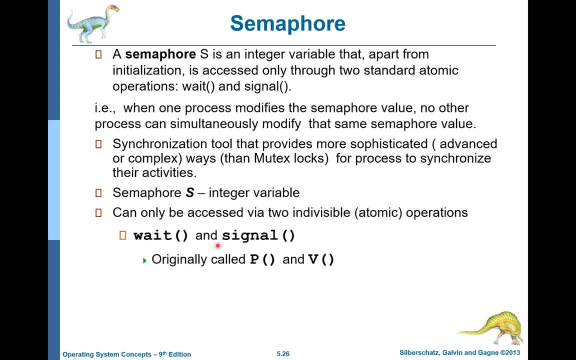 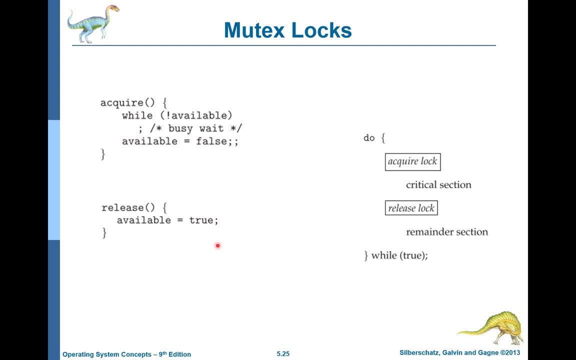 strategy of actually implementing the critical section problem, where we want to allow only one process to enter into the critical section. this strategy or this tool is called semaphore. okay, so before, uh, the lock in the last mutex lock, there was actually the acquire and release functions and there was one variable which was called available, which was false or true in this. 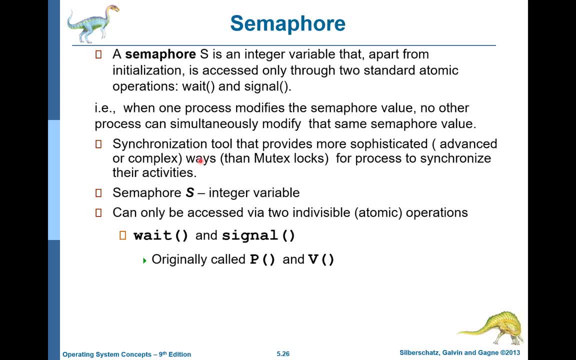 case. so so that was the available is actually a boolean variable. in this case, the semaphore is an integer variable, and this integer variable can be changed using only two operations, either weight or signal. okay, so they are similar to acquire and release, but in acquire and release in mutex locks 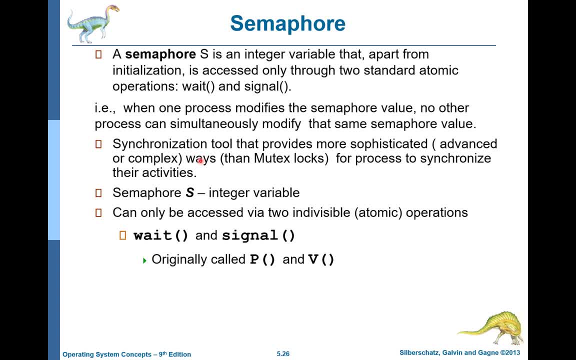 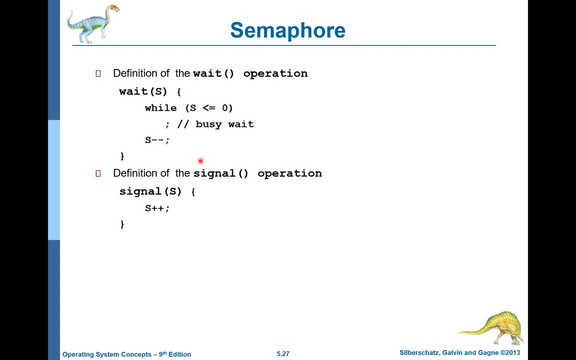 only uh boolean variable, true or false. here we can have an integer variable. okay, so it is better than or advanced than the mutex lock. okay, and because of uh it is an integer variable, it means we can also use it for more than um. i should say that if a resource has more than one instances, 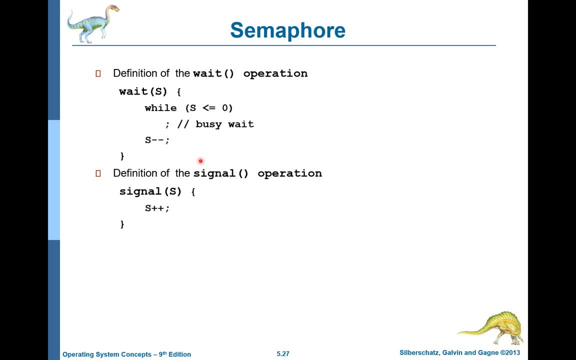 if let's say, instead of one thing you can have 10 things and you want to access the limit to these 10 things. so one by one, a process comes, it is using that thing or that resource and when all the resources they are finished or they are acquired, then you can lock the rest of the things. 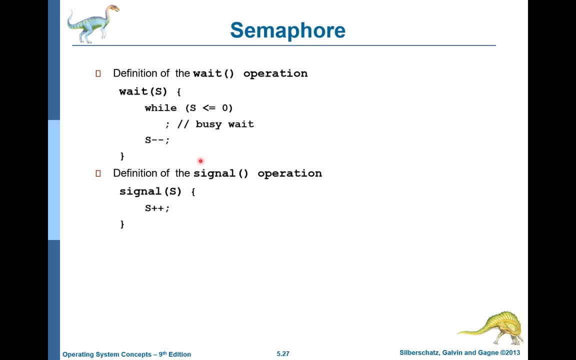 and the remaining processes. they have to wait to get those things. let me explain, okay, so we have two functions or two operations: one is weight and the other one is signal, and they have this s okay, for which actually? uh, you have to wait. this is the semaphore. 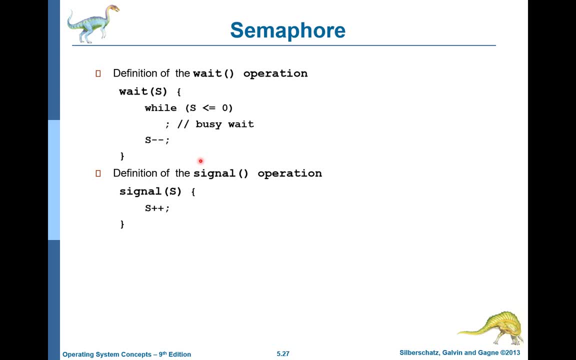 in the weight function. the purpose of the weight is actually to see if the critical section is available or not, and you do that again using this same busy weight thing. the value of s is less than or equal to 0. okay, then you wait if it is not 0 it. 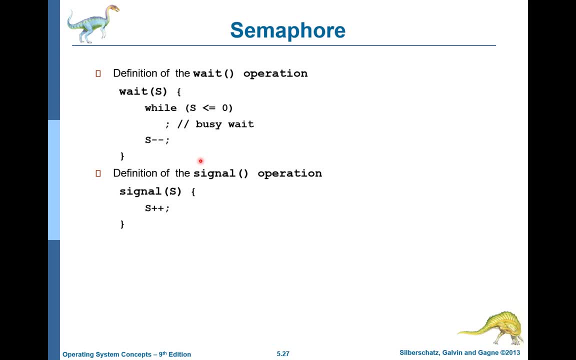 is greater than 0, then you decrease the value of s by 1. why we decrease? because we want to show that now this resource is used by me, so we reduce the number of available resources. if there is only one resource, it becomes 0. if there were 10, 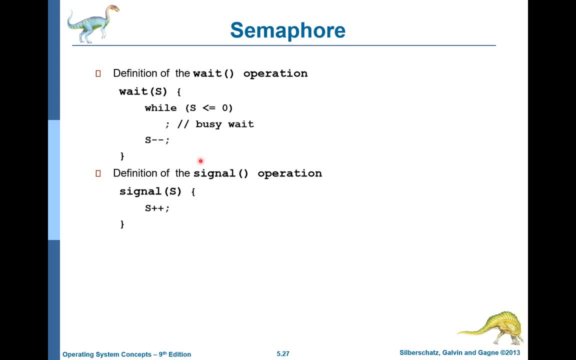 resources, then when you enter into the weight, then you make it 9. okay, so this way, reduce the available number of resources. when you do this decrementing of s, then you go out of the weight and you can go into the critical section. when you come out of the critical section, then you execute the signal. 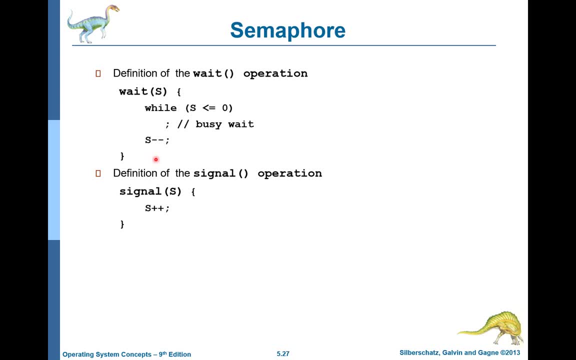 statement or the signal operation, which actually has only one statement, that is, s++, which increments the semaphore. why do we increment? because we want to show that the resource is now available. if there was one resource, in the weight it becomes 0. it was not available and in the signal it becomes 1, so it is available if there. 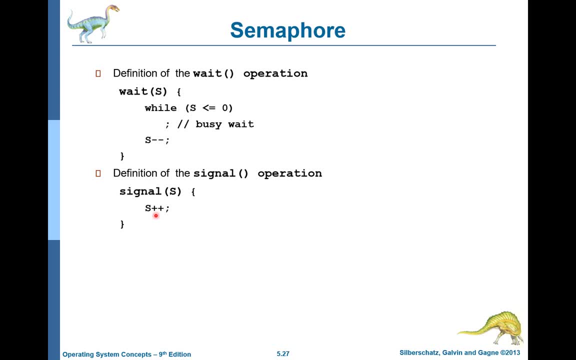 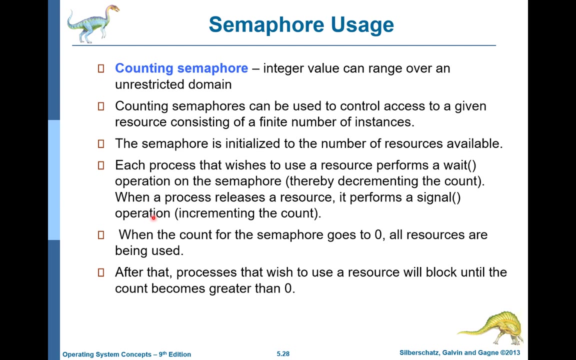 were more than one resources. so in weight you decrease the number of available resources, and now it's available because you are no longer needing that. so counting semaphores, as I explained before, is actually used for more than one resources and every time you initialize, you initialize it according to. 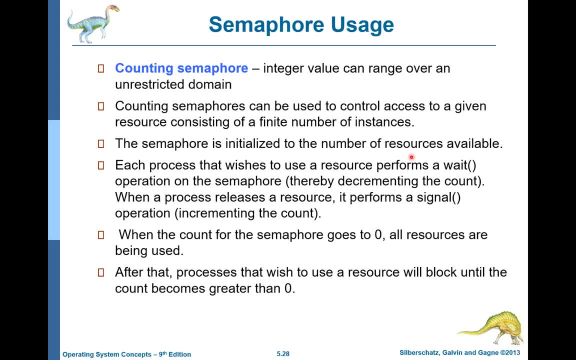 the number of resources, 10 resources, 5 resources or whatever. you do that, okay. and when the count for the semaphore goes to 0, which means that all resources are being used, then any more processes which want to use the resource, they will be blocked. ok, and any process which is in that critical section of the resource when it 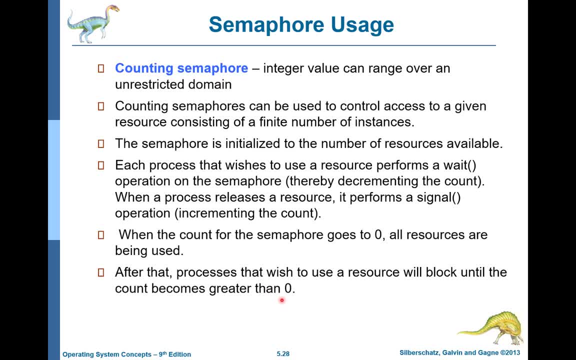 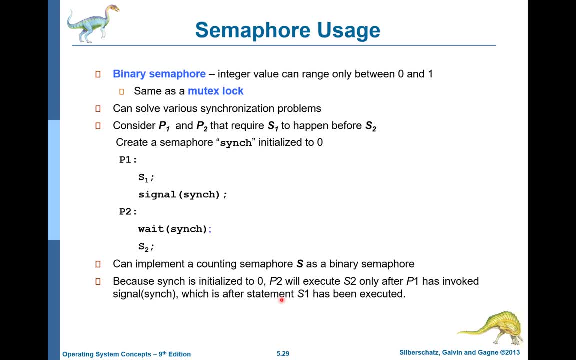 goes out, then the semaphore is greater than 0 and any of the waiting process, they can use that resource. ok, another, so this is this was the counting one and in the last slide and this one is the binary one. ok, the binary one can also solve other type of synchronization problems. 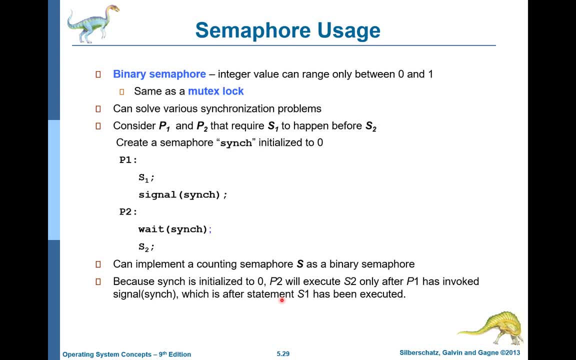 for example. here we can see, if you want that s1 must happen before s2, okay, s1 is some process or some statement that must happen before s2, okay. so in p1 we want to make sure that s1 is before the signal and in p2 we must make sure that. 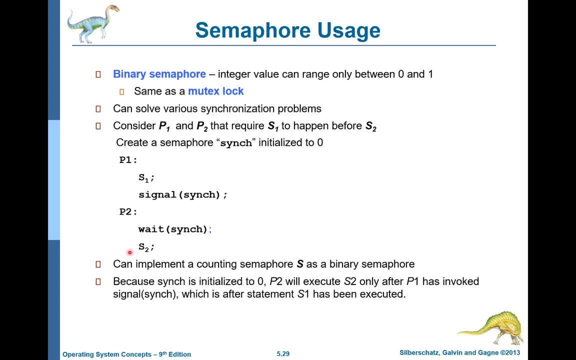 s2 is up to the signal. so this p2 can never execute s2 unless s1 is executed by p1. why? because it is waiting for the sync. okay, and here this is the signal of the sync will be released after using s1. so when s1 is used and this process 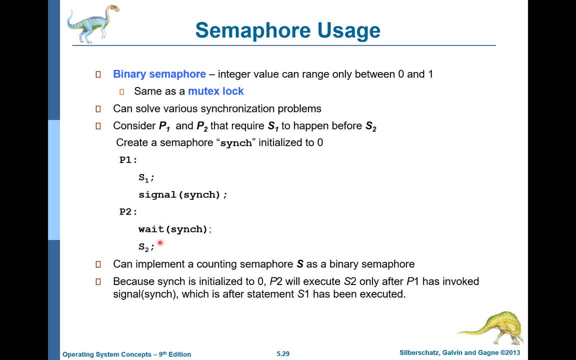 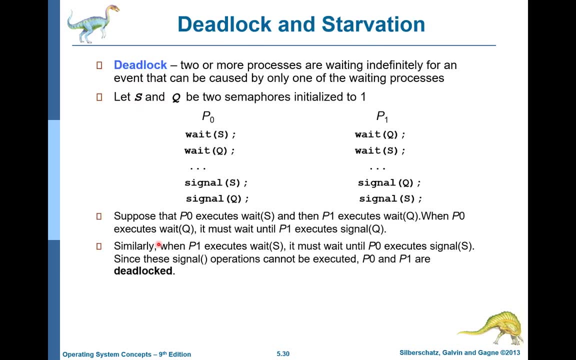 signals sync, then it's can go into wait, sync and execute s2. so this is very interesting use of semaphore. also, we see that these semaphores if you use for more than one resources, then it can create a problem which is called deadlock. okay, what is a? 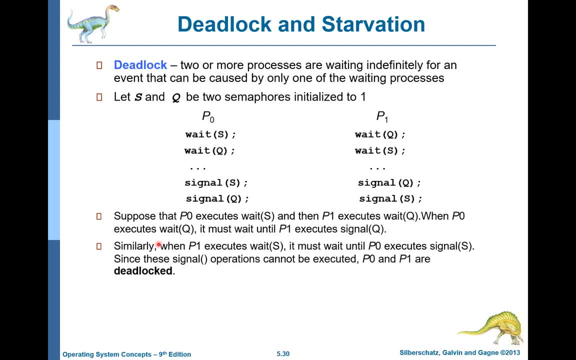 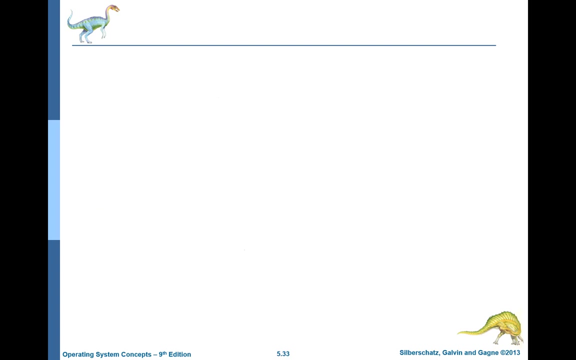 deadlock. a deadlock means that when two or more processes they are waiting for something which is not available or which is only accessible if one of the waiting processes does that operation. let me give you an example. let me explain that with the help of an example. so let's assume to explain to you. 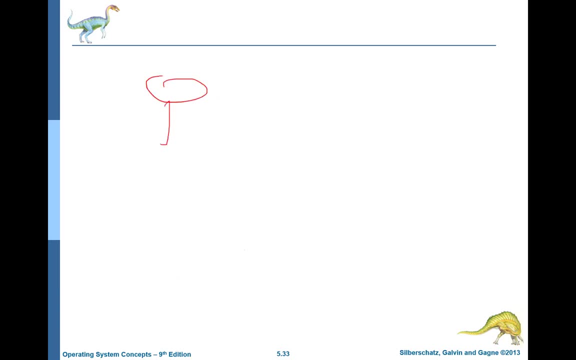 the process of deadlock. let's do. let's assume there are two people. okay, two different people. maybe these seems like wise, but you can say: these are boys, start, goes and each one of them wants to write something on a paper. okay, so there is some paper. and then there is only one pen. okay, so they want to write something. 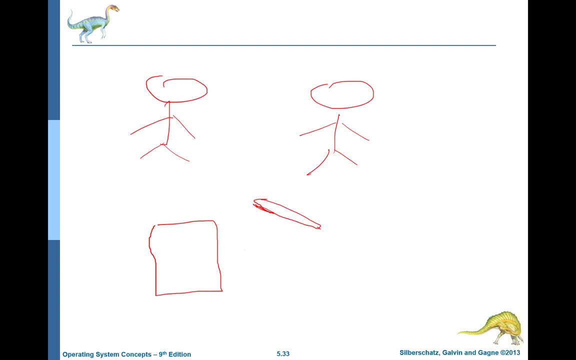 on the paper with the pen. if this person here on the right it gets access to the pen and the paper, he can write something on it. or if the second person gets the pen and the paper, he can use them. okay, but for anyone to use it's important. 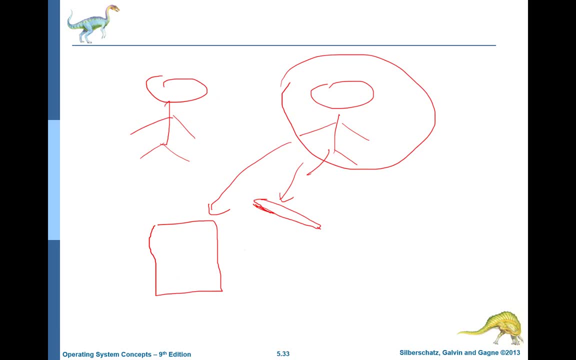 that they have access to the pen and the paper at the same time. now assume that what happens is that, let's say, this person, one of these persons, he gets the pen. if they will send lá change, there will be letter from the federal government to this person, which means that one of them wants to use the pen and the paper. 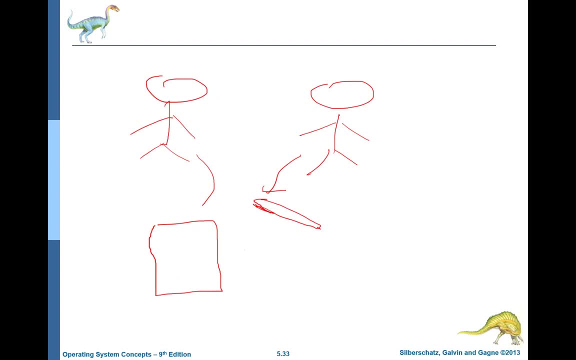 okay, this person gets the pen and this person he gets the paper. now how can they write? they cannot why? because this person is waiting for him to give the pen and this person is waiting for the other to give the paper. they are waiting for one another. they have the resource, each one of. 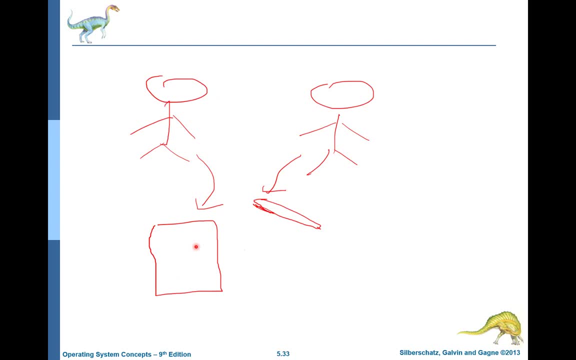 them has one resource, but they are waiting for the other resource, so they cannot do unless they have acquired both the resources. so this is a deadlock, which means that in order to execute the- their action to write on the pen, each one of them needs to have access to both paper and 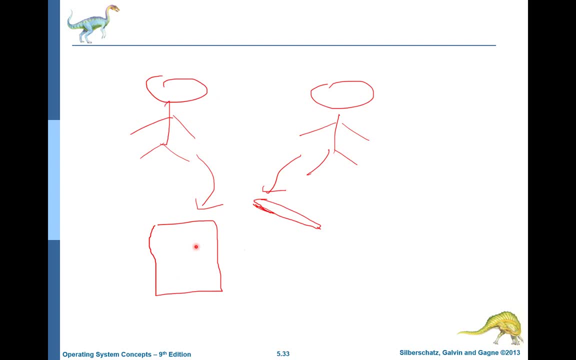 the pen at the same time. so how can we resolve the deadlock? that's something which is an interesting problem, but we don't discuss the resolution of a deadlock. the important thing is just to understand that actually, here we have more than one resources- okay, and any process which holds a resource. 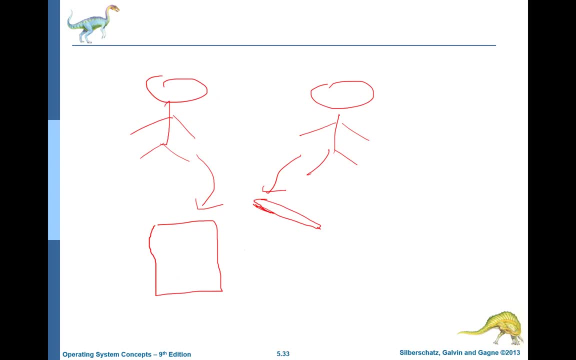 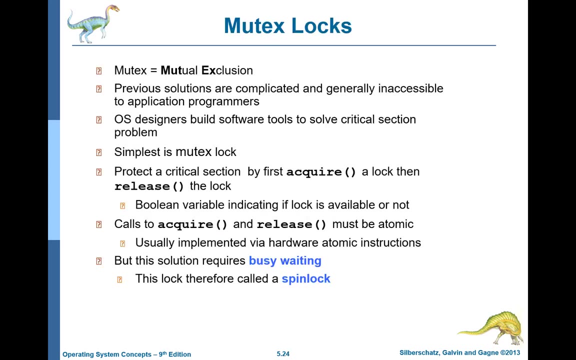 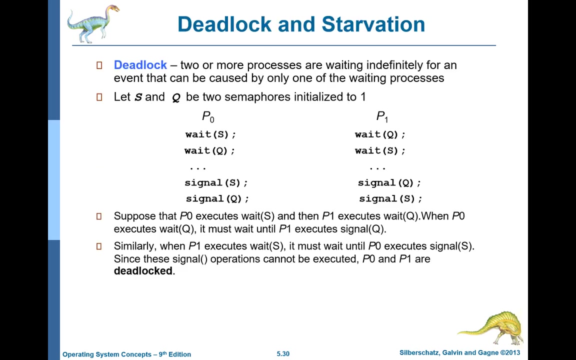 is waiting for another process to release a resource. this is called a deadlock. do you understand this okay? so that one is this process, when many processes, they hold different resources and each one of them is waiting for some other process to release the resource. so here is the example that let's let s and q be two semaphores. 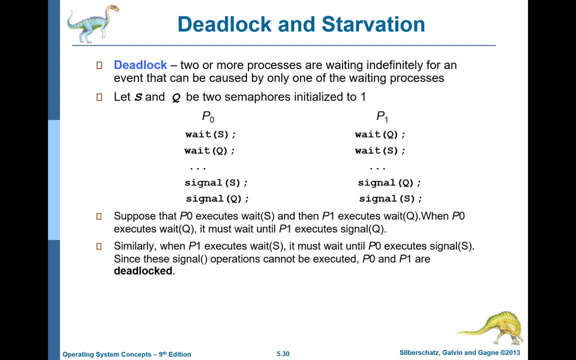 okay, and we initialize them to one here. okay, and what we want is that in p0, let's say, we want to access some resource s, and in p and after s, we want resource Q and s and Q. they both are one, which means that there is only one resource for semaphore s and only one resource for. 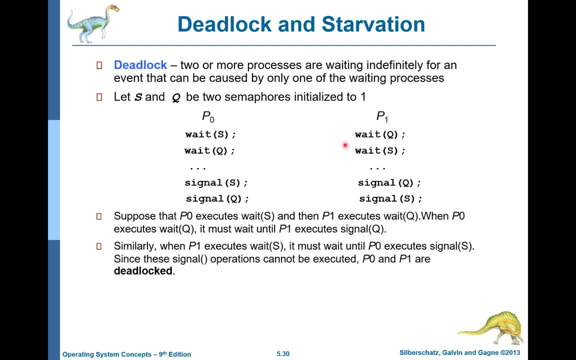 semaphore q. similarly, p1, it gets access to q and it wants s. what is the problem here? when this one, p1, it gets s, it tries to get Q, it cannot because Q is being logged by p1. so p0 is waiting for q and p1 it has got access to q, but now it is waiting for s. 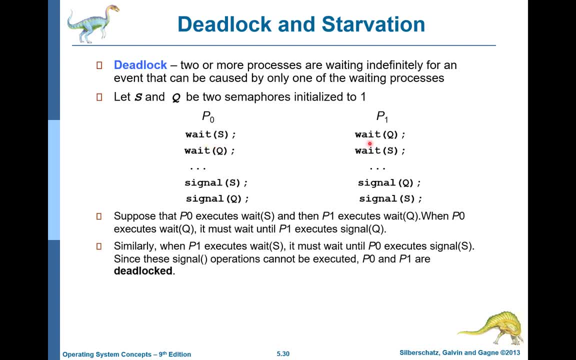 so s is held by p0 and q is held by p1. p0 is waiting for q and p1 is waiting for s, and in this way, they both are waiting for each other. none of them can go ahead. they are just waiting forever, and this is called a deadlock, okay, so this deadlock needs to be solved and 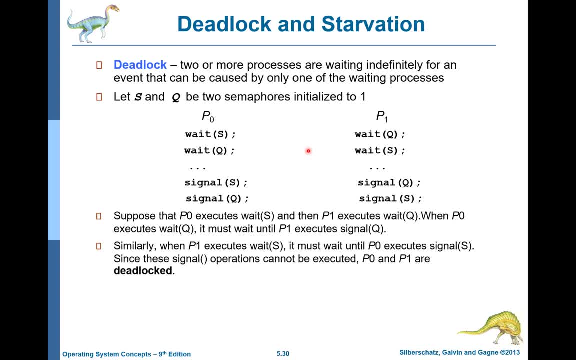 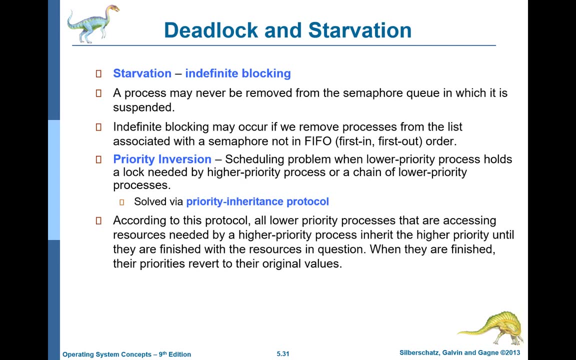 there are different procedures which are there to avoid deadlock. okay, it should not happen at all, but we are not going to study this in this course. you just need to understand what is a deadlock. the second thing is about starvation. what is starvation? starvation means you are robbed for. 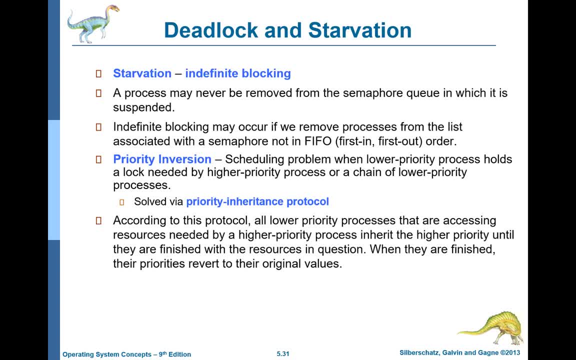 something you for a long time. okay, why it happens? it is because you are waiting for something and maybe sometimes soon your number comes. but then there is another process which comes before you and he gets treated before you. this happens if you have q, but in which you do not actually enforce the first in first out. 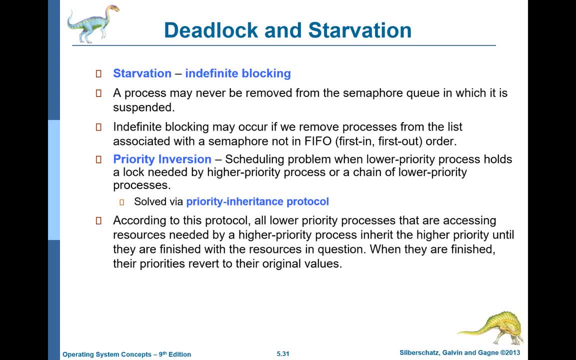 so if there is no first in, first out in the queue, then it means any person or process can come before you and they will solve their problem and you will keep waiting for an indefinite period of time. if the q is first in, first out, then there is no problem. the first process comes it. 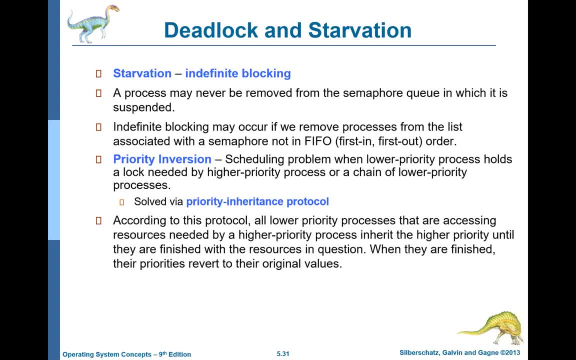 goes out. but if it is not first and first out, then it means that the one who is in the last, he will keep waiting because new processes will come before it and they will execute and this will keep waiting. one other problem is that of priority inversion, because let's say, in the queue, if everyone, so what happens? 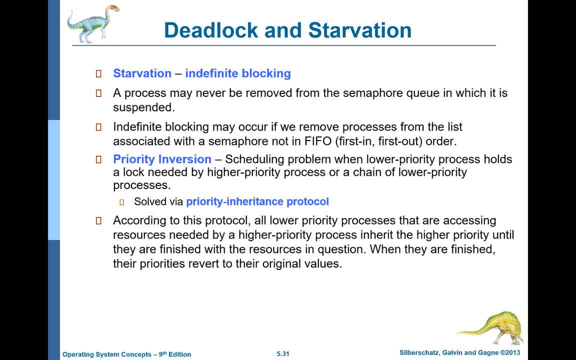 in the case when the first in, first out is not implemented, it means that some process has more priority. this happens, then, that when a low priority comes in the queue, but after the process is inside the queue, new processes with higher priority come. so they go in the front of the queue and they are 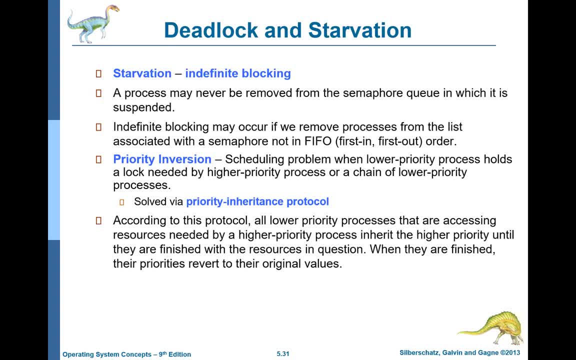 executed before this one. so before this turns comes the other processes, they are executed and in this way it keeps waiting for long and long. how can we do this? we can have something which is called priority inversion. this happens is that sometimes the low priority it goes into some lock, okay, and then the higher priority needs higher priority. 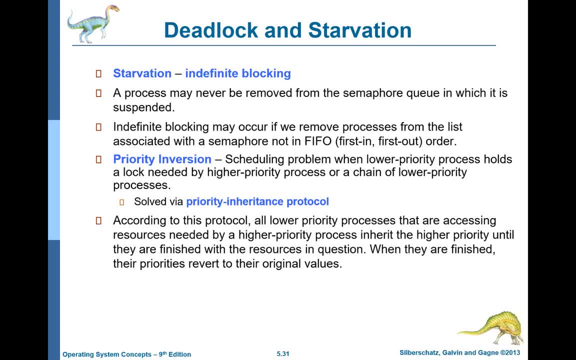 process needs that lock, but because of the lower priority chain it cannot access. so this is also a type of starvation, because higher priority must be executed first, but because the lock is held by lower priority, so it cannot execute and it has to wait for a long time. 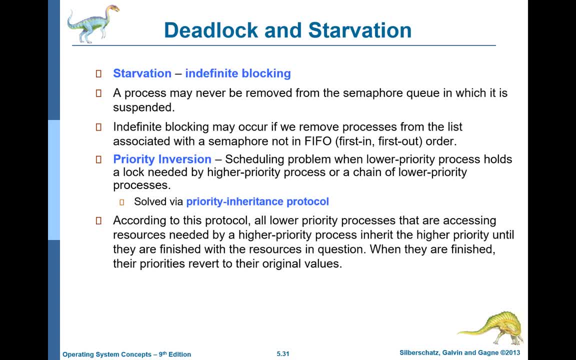 if we implement something which is called priority inheritance protocol, then this problem can be solved, which means if a low priority holds some resource and there is a higher priority process which comes and wants that resource, so we increase the priority of the low process and give the resource so that it. 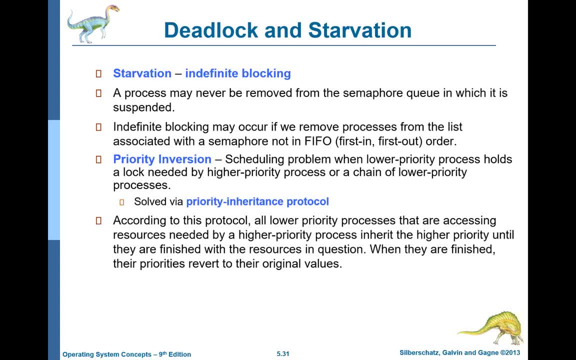 can be doing the process very quickly and release it, and the higher priority process can access that. now, if you don't understand this, no problem, because you are going to see this in the assignment. in the assignment I will ask about this and you are going to study the book and give me back the answer and then you will understand what. 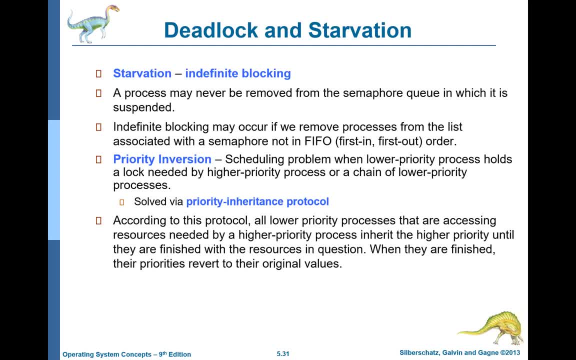 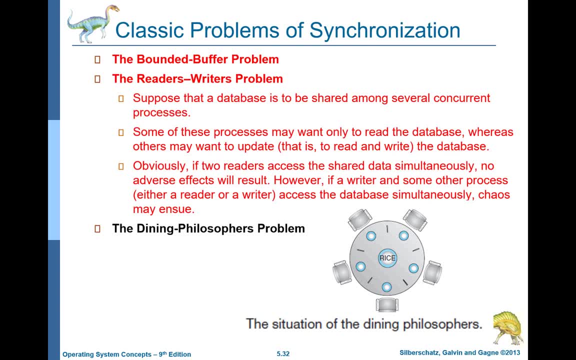 are these priority inversion and priority enhancing inheritance protocol? the final slide is about the classic problem of synchronization, which are there in the book. i am briefly explaining the first two. in fact, the first one we have already seen the bounded buffer problem. it is the same: consumer, producer, consumer problem. okay, so producer. 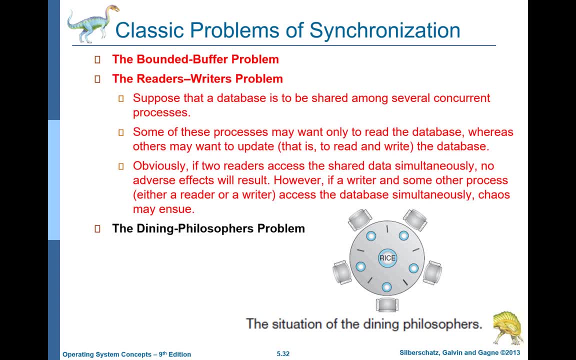 it produces something and consumer it consumes something. okay, and the synchronization is for the variable counter. you have to synchronize the axis of the producer and consumer such that there is no inconsistency in the counter variable. the second thing is about the reader writer problem. what is the writer problem? let's say there is some database and different processes they want to. 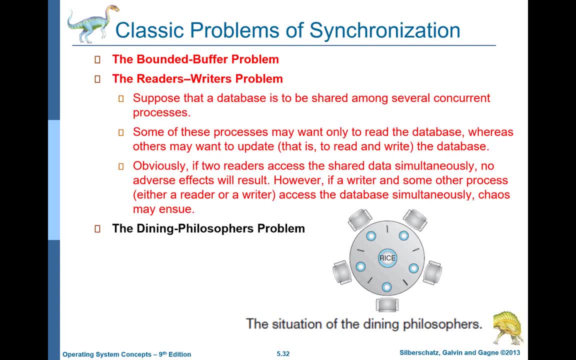 access the database, they may access it at the same time. if all those processes which access the database at the same time, they are only reading the value from the database, that is not a problem, because it does not change anything in the database. okay, you are just reading the value, you.